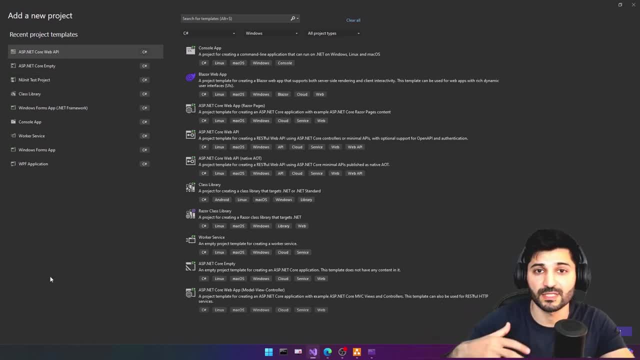 use them. But for me it is really easy to explain things from the ASPNET Core web API perspective because we'll be developing. web APIs are popular nowadays and also for ASPNET Core web API we have built-in Dependence Injection that will help us to not to write things from scratch, but easily inject. 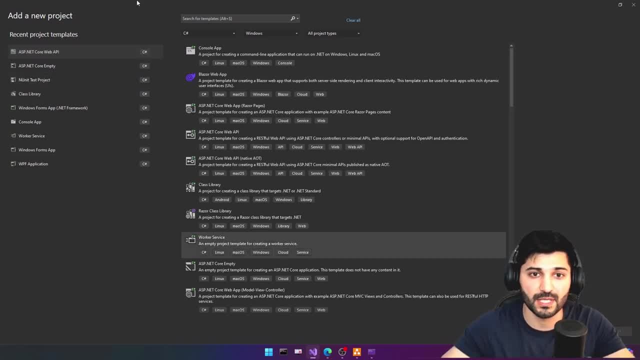 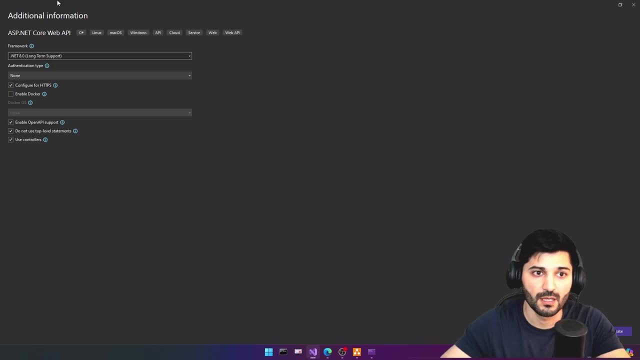 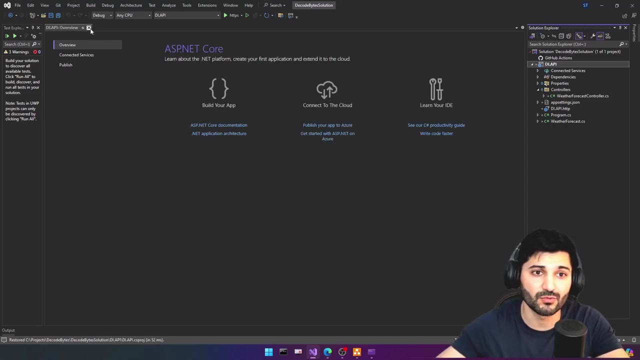 our dependencies. Okay, let's select our ASPNET Core web API. Let's create our project. It is going to bow at diapi, Okay, And I'm not going to change anything from here. Just use classical controller mechanism. What we're going to develop this is a really simple application. This is I'm 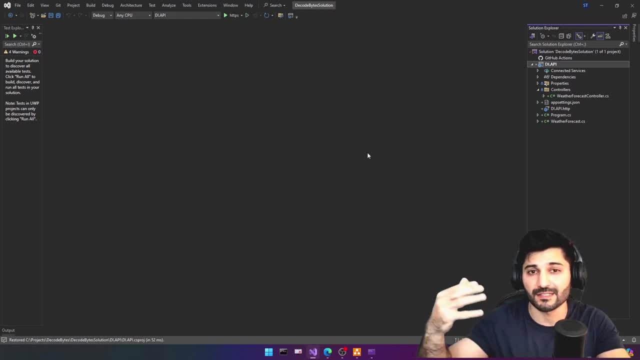 not going to use layered architecture. I'm not planning to make things really complex to show that I know everything. I'm just going to explain Dependence Injection. For that reason, I will have only one simple project and it is our API. All the layers I will add as folders. Okay, This our project. 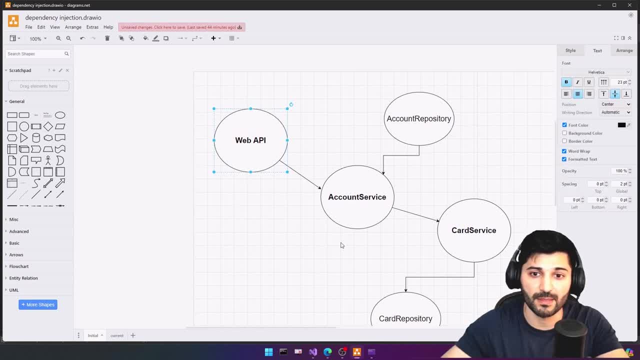 what we're going to implement will have web API. in our web API will have dependency from account service. For account service, we will use account repository. As you know, they are just real, exact implementations. We are not going to use interfaces, abstract classes. 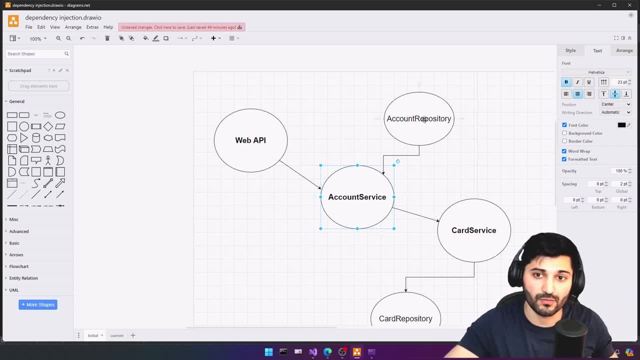 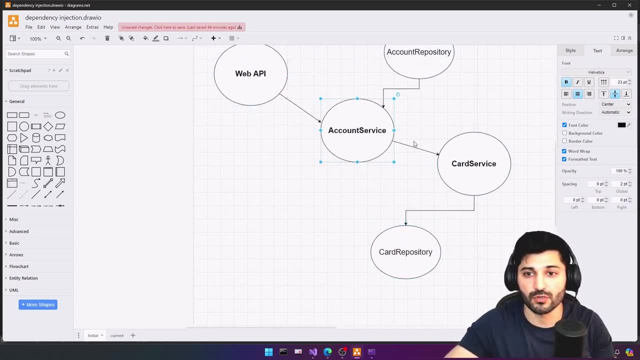 we'll have direct implemented service called account service. It has direct dependency from account repository, card service and card repository. Our web API will use account service and our account service will use card service. I'm just going to show you what is the problem with using this approach. Of course, sometimes it is better to not to use Dependence. 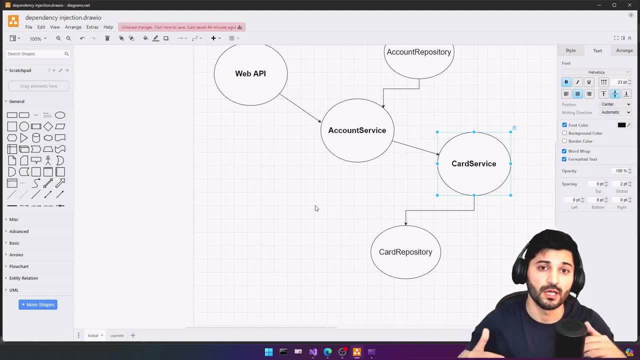 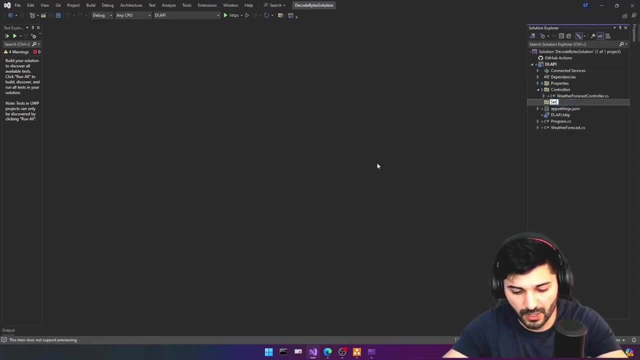 Injection, because Dependence Injection is also can make your life hard, But in some cases it is better to rely on Dependence Injection. and let's fill it together. Okay, Great, I'm going to have add new folder. This is our services folder, This is our services layer and we'll have another. 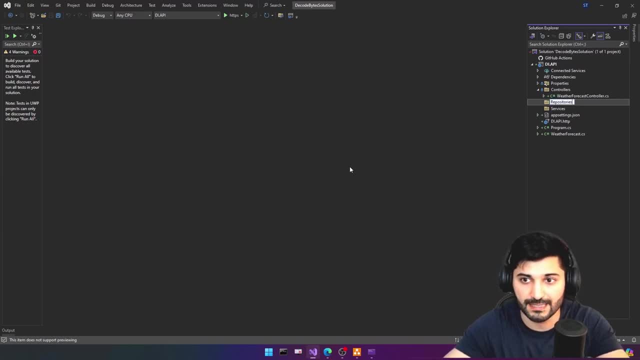 layer called the repositories. I'm going to implement the implementation and contract stuff inside these folders And of course we need some sort of models. here again, models: I'm not calling domain model because I will not write domain model, I will just provide the Anomic model that 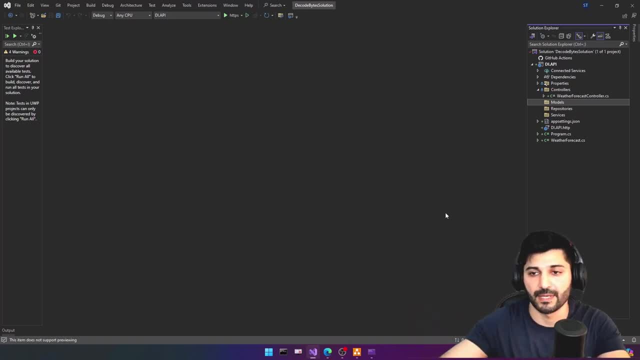 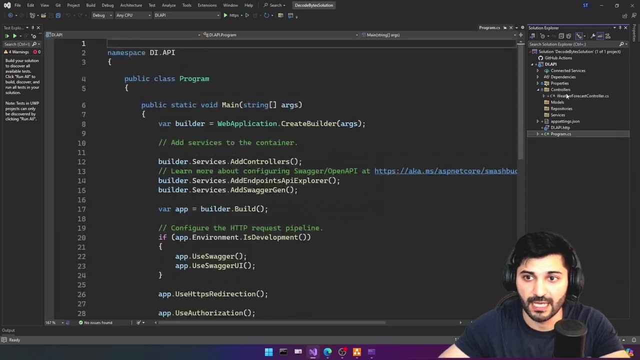 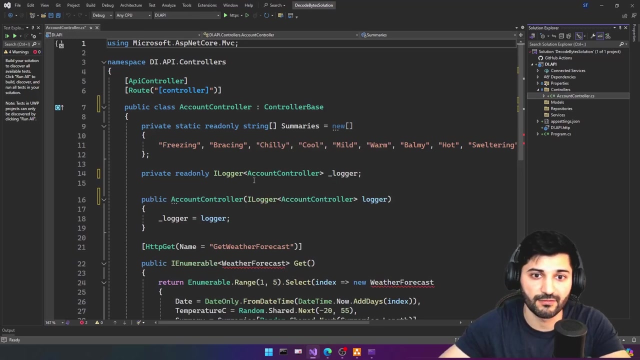 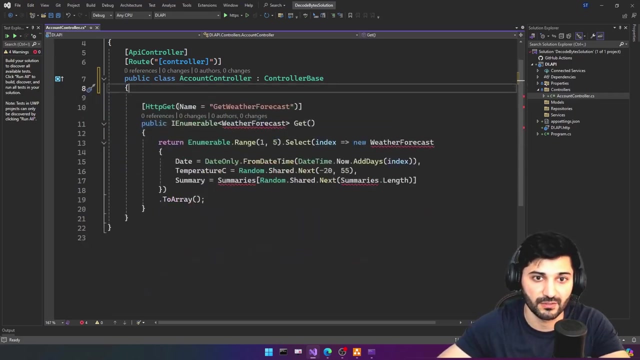 will help us to work with database. Okay, Great, Let's remove our weather forecast here first And let's rename our controller to first account controller And for account controller. I don't need this information And, of course, let's completely remove all this stuff here. 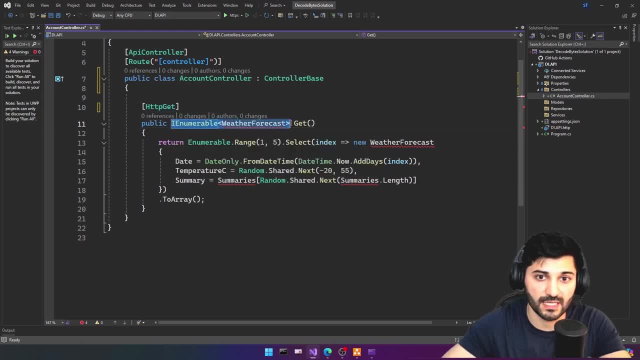 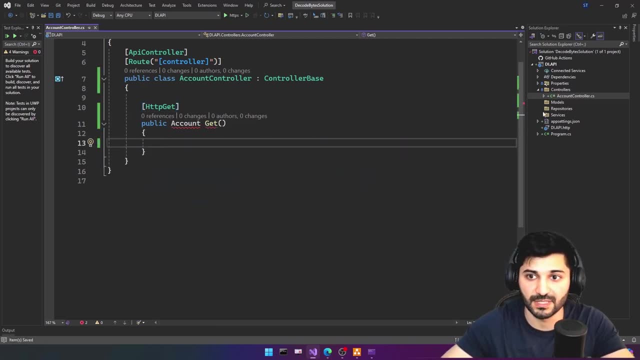 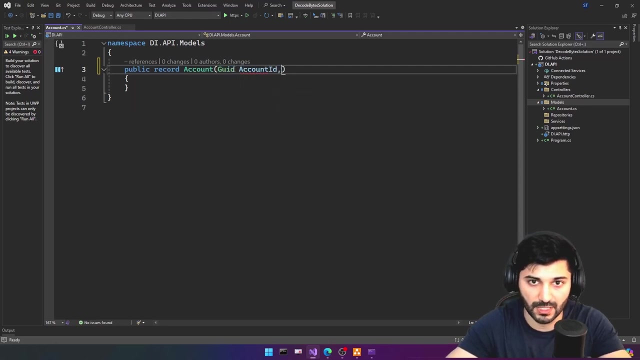 Let's remove this name and we'll just simply may return account information And that's all this, our simple template. I'm going to have our model folder account. This is simple account which is going to be our record And it has just simple account ID string, account name and, of course, 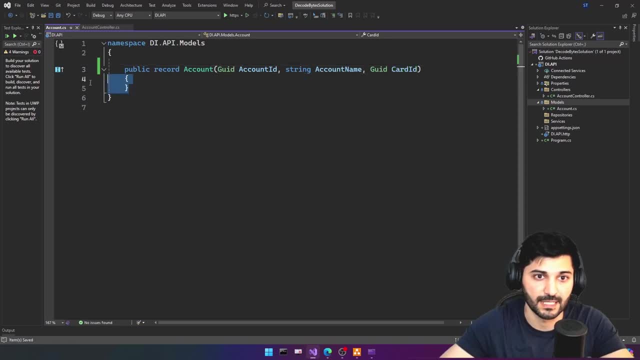 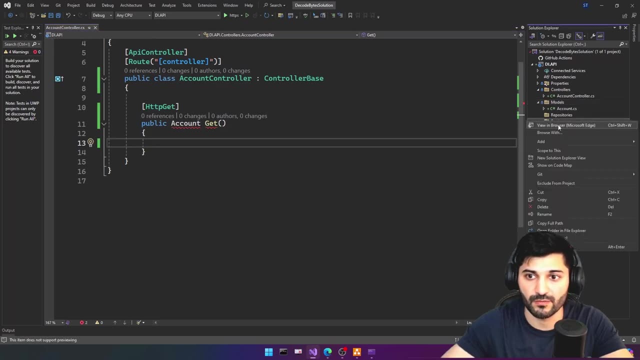 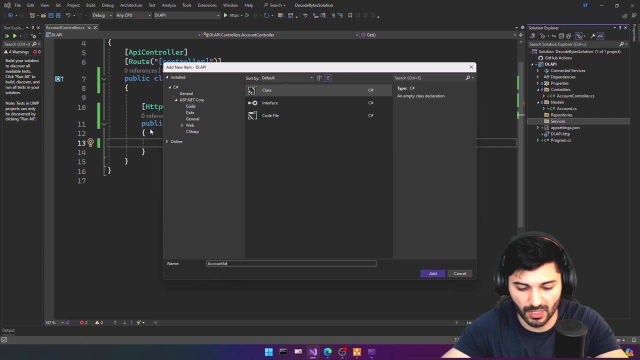 grid Our card ID. That's simply okay, I guess. Cool, And now let's go to our services. right click. we talked that we will directly implement our account service. For that reason, I'm going to have account service And in my account service I will have a simple method. 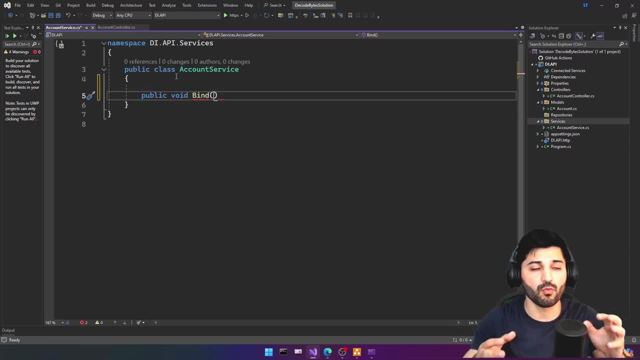 called bind. The purpose here is: I want to bind my account to, to my given card. iI have account information. i have card information. I want to bind this card to my provided account and do it account ID and do it caught ID is. 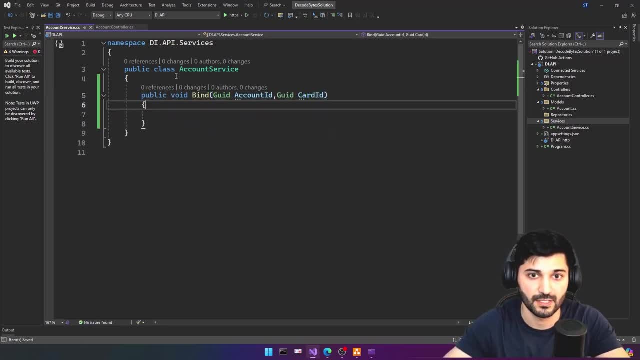 our going to be our arguments in this case. great, What we need to do? first, of course, we need to check if we have this account information. this a classical approach. I'm not going to dive into details. so you have some sort of repository here, let's implement it. add new class. 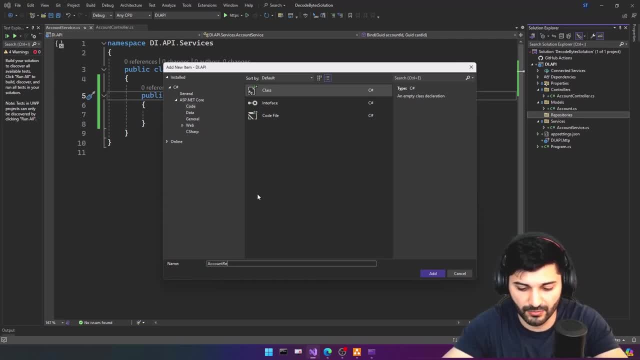 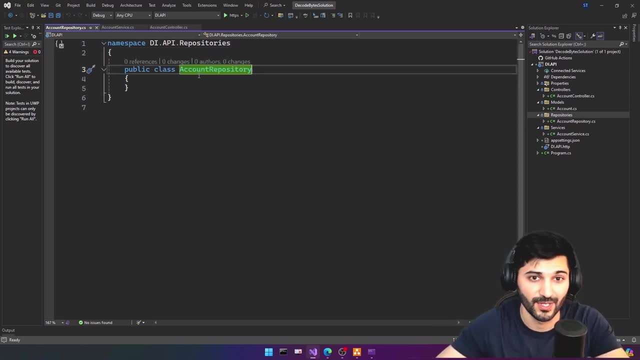 so you're always doing something like this account repository. okay, this is your repository. you really love to create leak obstructions, so we have a counter repository here and public account information. get account by id and, of course, uh, for the repositories, we always have asynchronous operations: task account and grid account id. we'll just check our account. i'm not going to integrate. 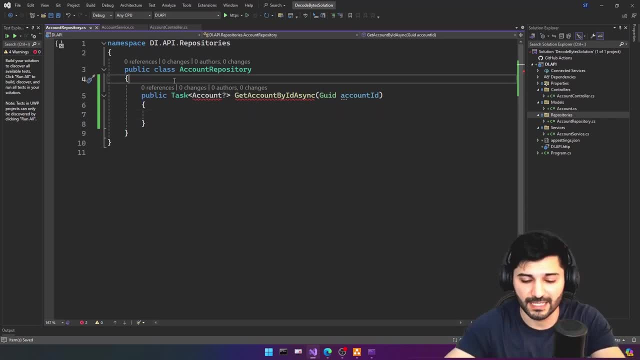 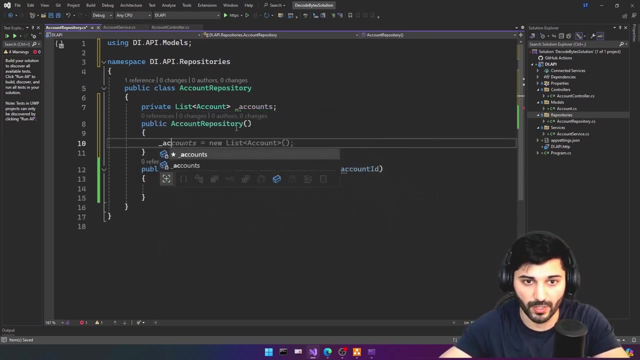 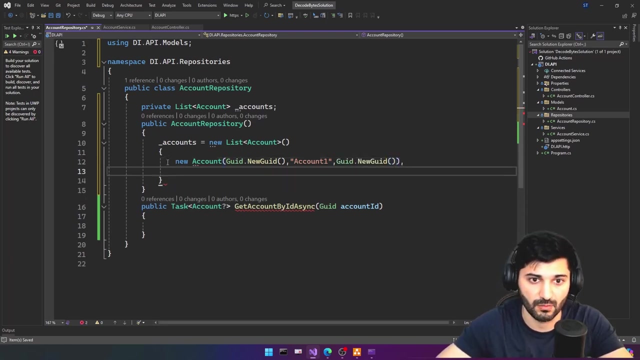 into the framework. for that reason, i will have simply in memory data structure and private list account and this is my accounts. okay, and from the constructor i am going to instantiate some account information. new account: first, let's randomly generate it and let me just copy this stuff because i will use it. and account one is going to my account name and this one also is our. 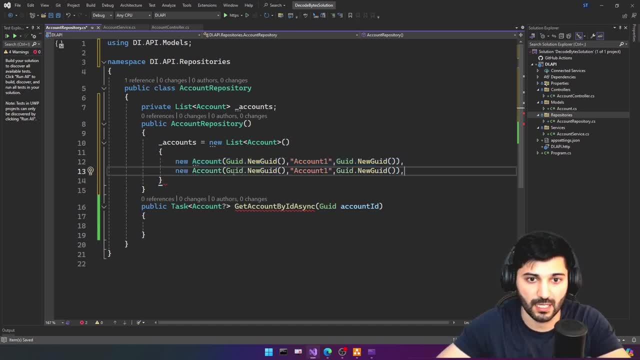 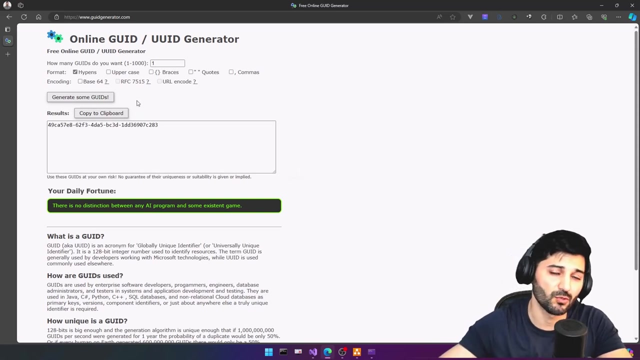 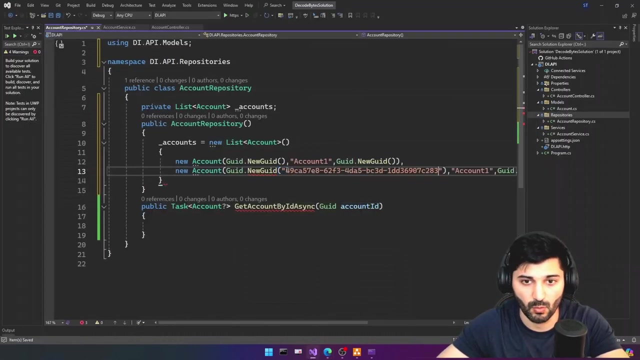 card id. and next one is our next account, which i'm going to use already generated grid value to search things really easily, let's just copy. so you see, we have a lot of uh online websites that help us to generate give it, so i'm just able to copy one from here. let me just 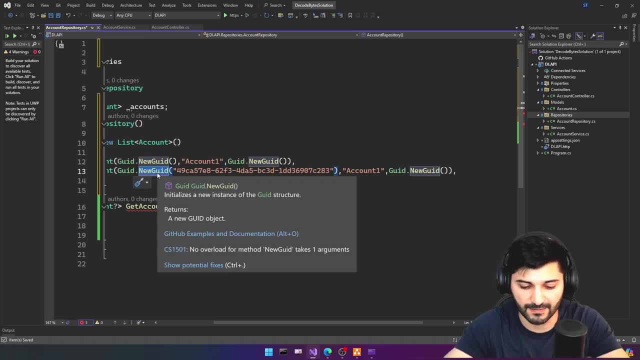 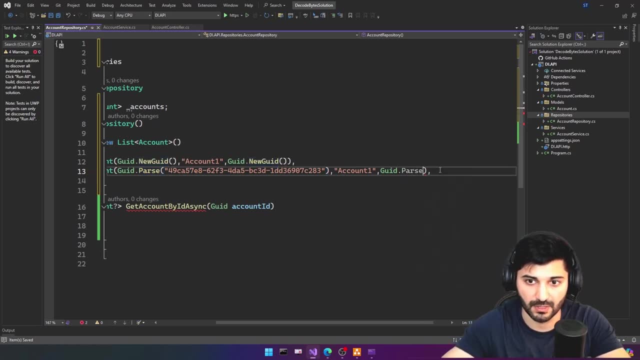 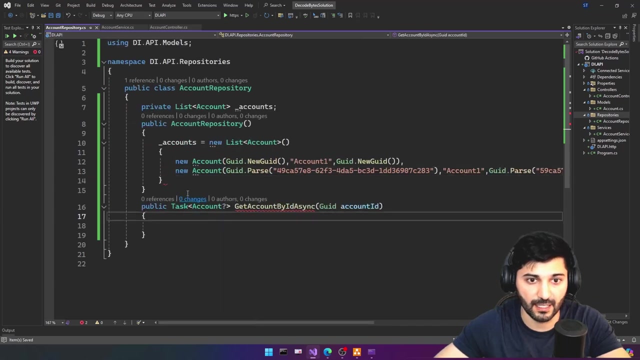 copy it from here. this is a give it that not near id, but parse, and the same stuff is applicable here also. let's just copy this stuff and let's paste it here and it will start with five: cool, and now we are able to search for some value return accounts. 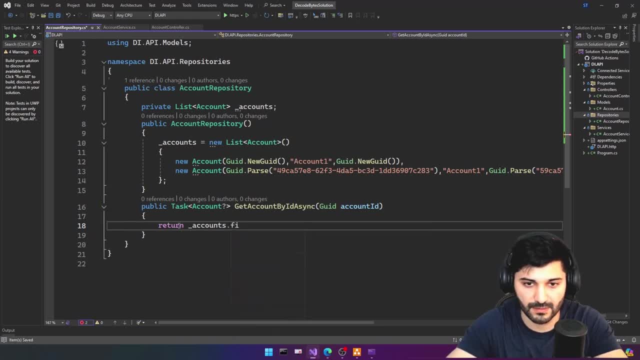 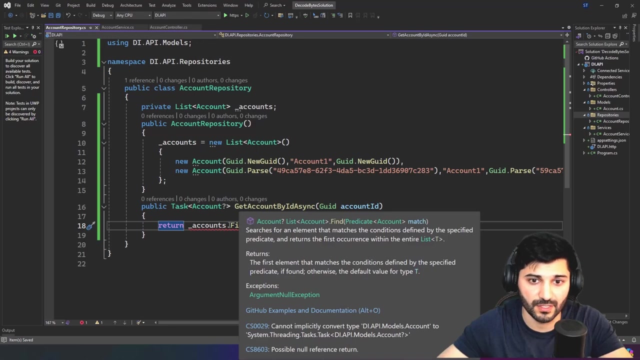 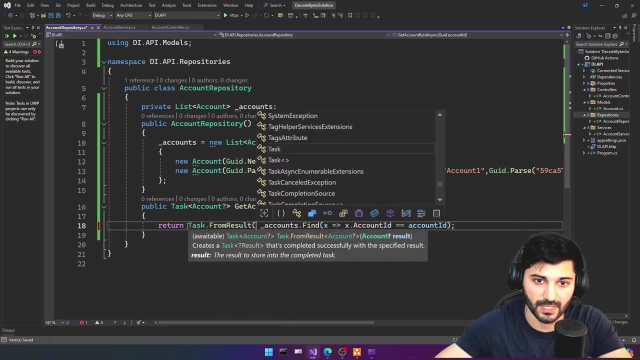 a dot. um, let's use, i guess, find, right now find and let's provide our account id to account id you can use in other methods. here it is completely okay for us to use it, because right now it doesn't matter for us the optimization stuff and etc. from result and that should be okay for our 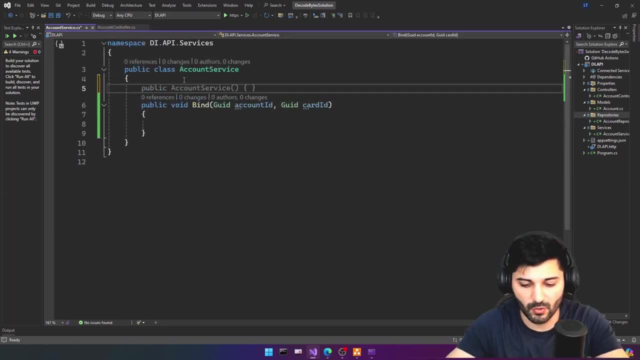 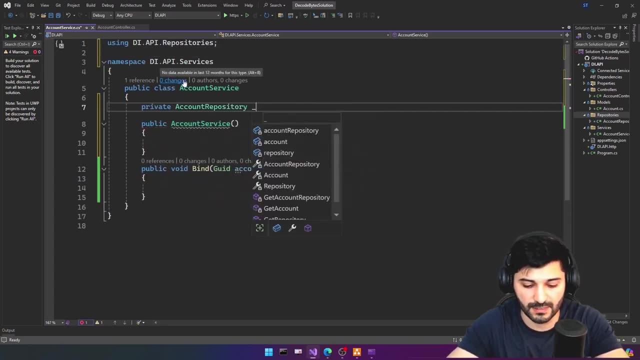 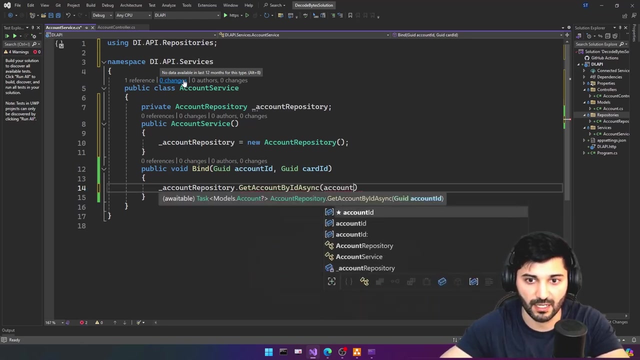 account repository and for the account service, i'm going to have our repository, private account repository. this is my account repository, okay, and i am instantiating the exact instance of account repository. and for the account repository, i'm going to check if given account exists or not, and this is going to be task async operation and here we have await war account. 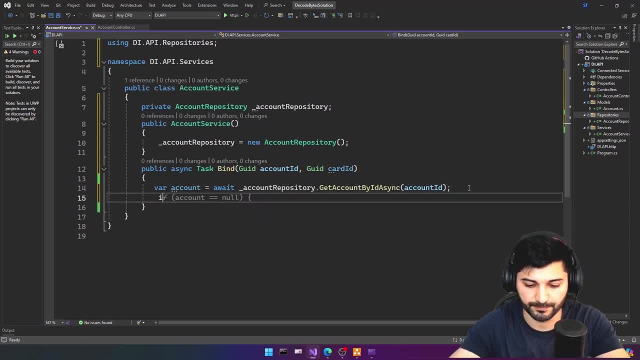 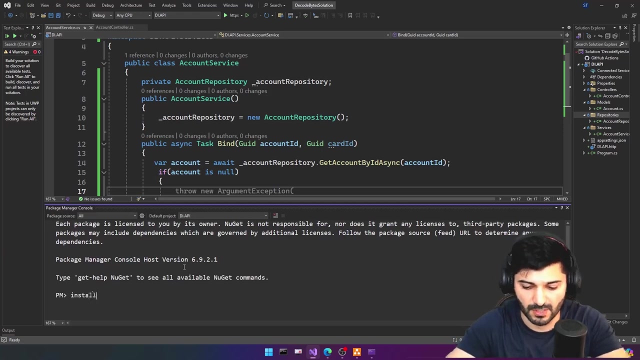 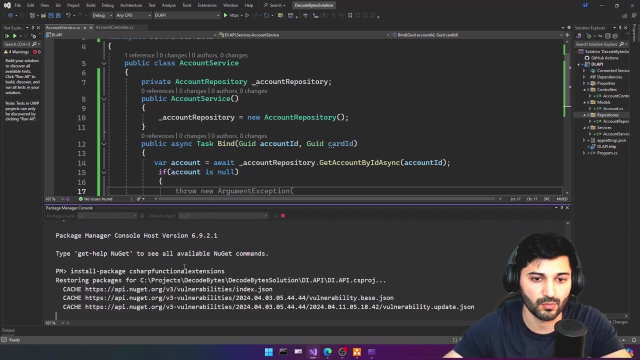 information, that's okay. account okay. if our account is null, then we'll return some information. for that reason, let's go to tools, uh, to do new package manager, package manager console. i really love c sharp functional extensions. install package c sharp functional extensions. let's install this one. 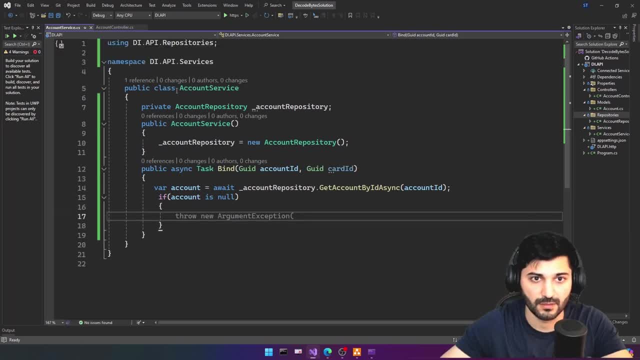 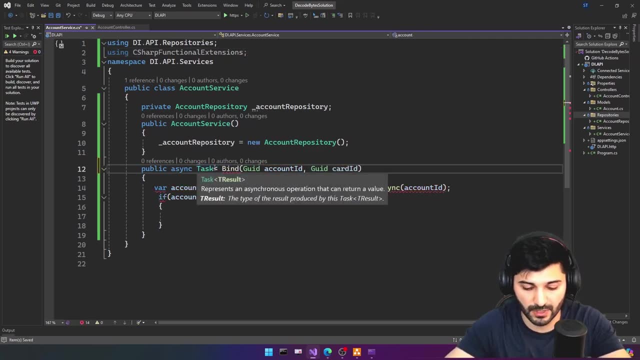 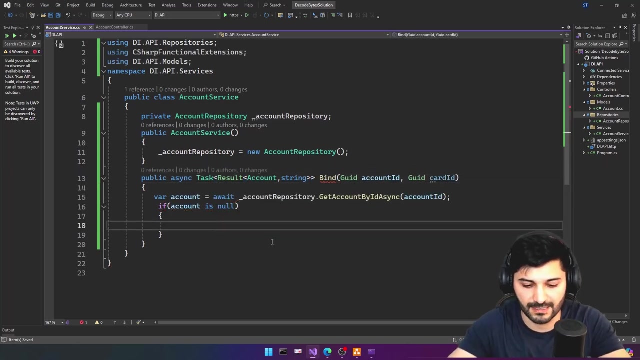 so let's see, using c sharp functional extensions, i will return uh, some sort of release result here. so the task result: account and string: error. okay, if account is null, then return result: dot failure. and this is my account string: no valid account id provided, great, and else we'll check our card id. we'll use approximately same operation here, okay. 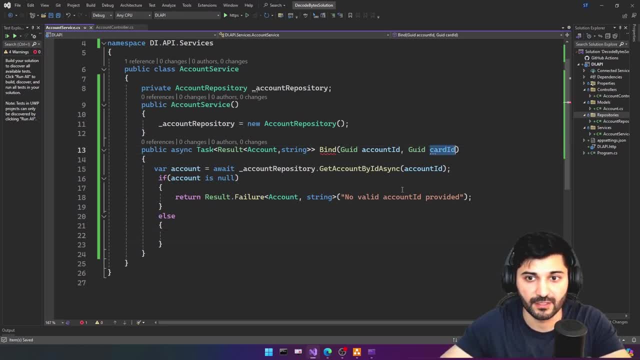 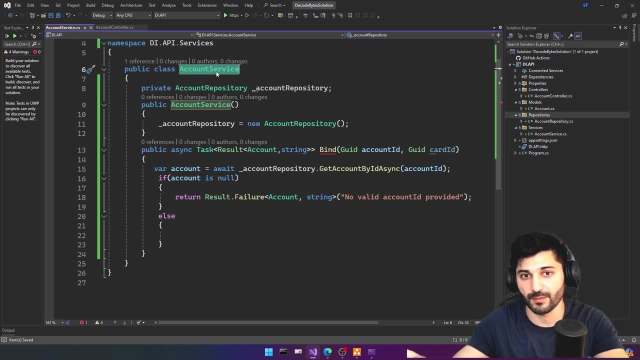 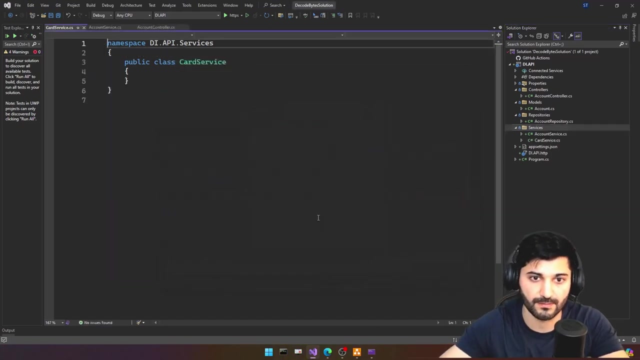 so i am going to have card service first, because in my account service layer i will interact with not card repository but with card service, because for card service we will have additional business logic stuff. so let's right click, add class card service. okay, and for the given card service. 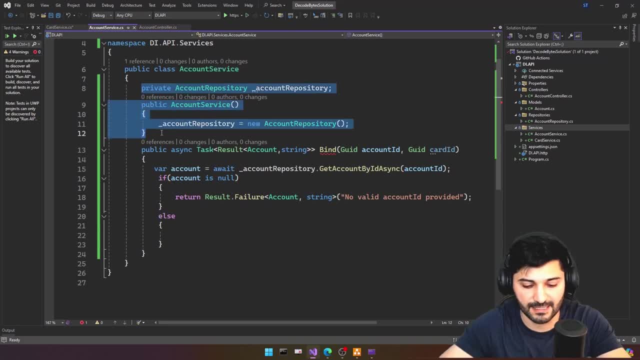 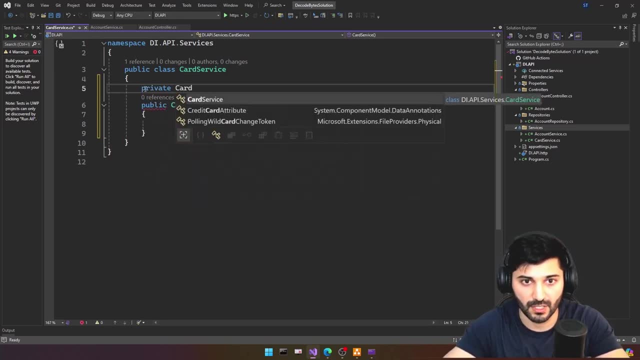 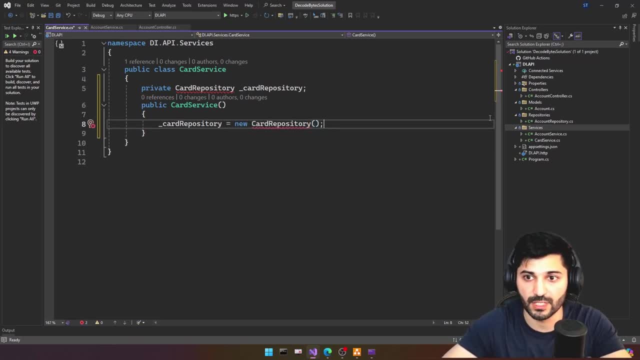 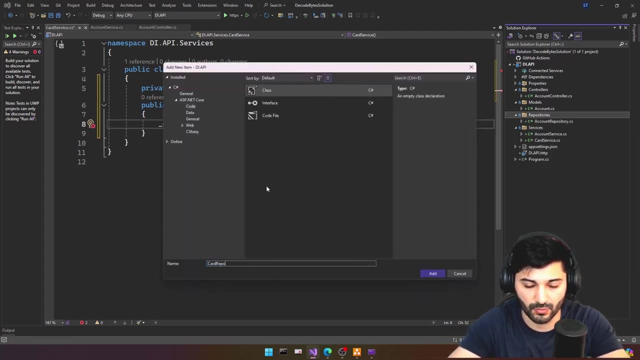 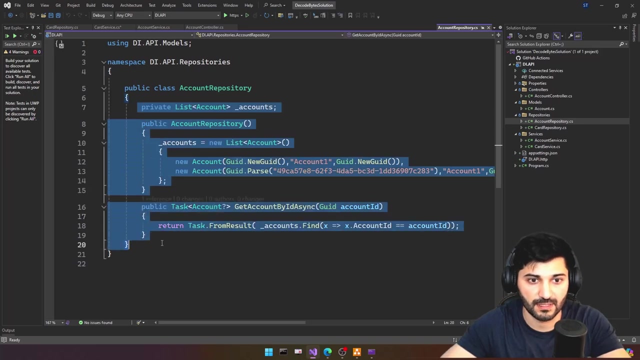 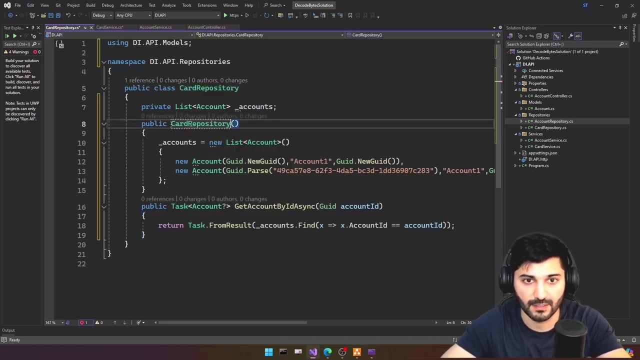 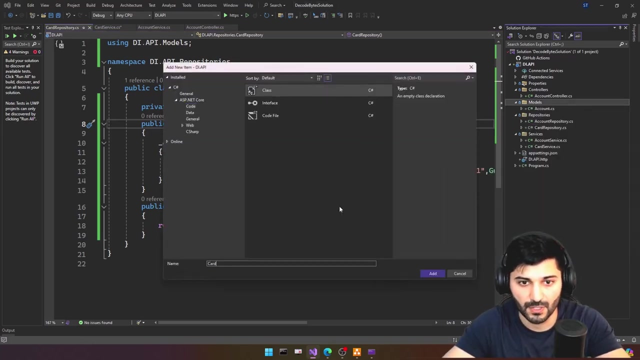 and we have a card card. cool and repository, new card repository. let's go to our repositories, right click class and this our card repository, your lovely repositories, and let's just copy this stuff from here, paste it here: card. let's create a simple card here: right click, add class card. this is going to our record and 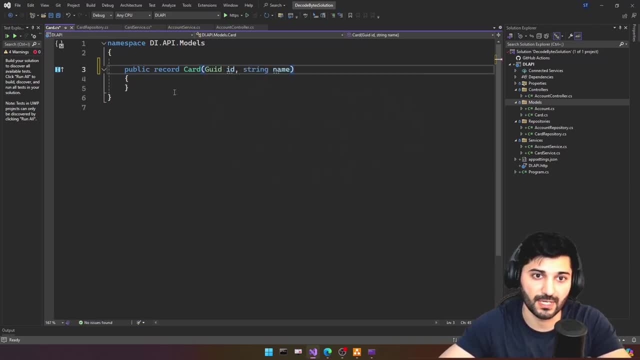 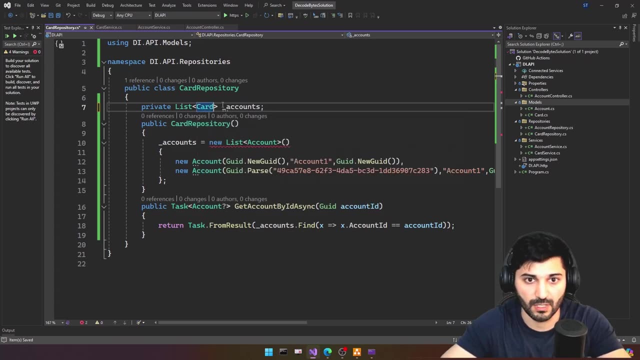 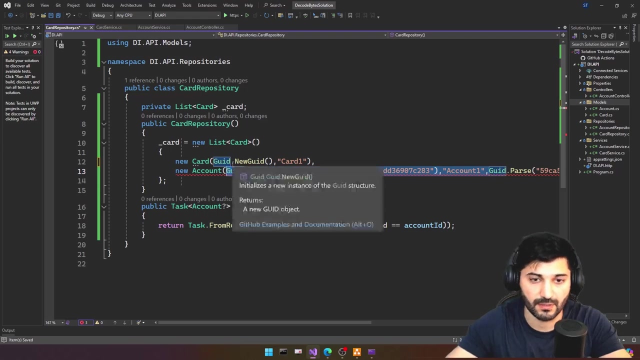 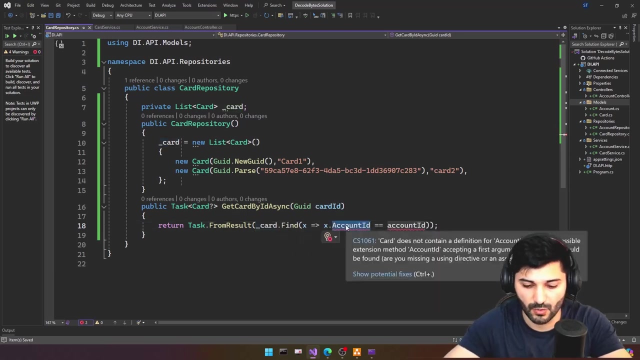 grid: card id, string card name. that's enough. okay, and this is our card. this is also a card card, new card, new card with card one and, of course, card two. great, this is my cards and i will return some card information. get card by id card id and from the cards we will search for id card id. 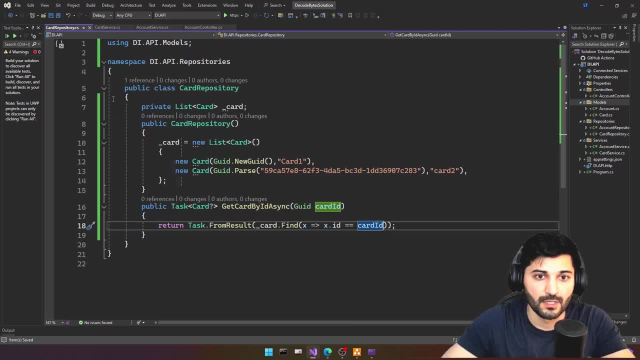 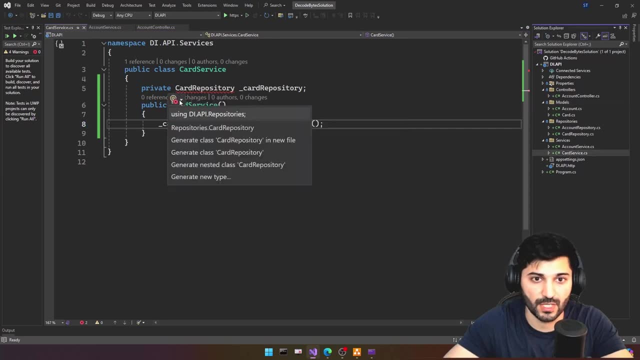 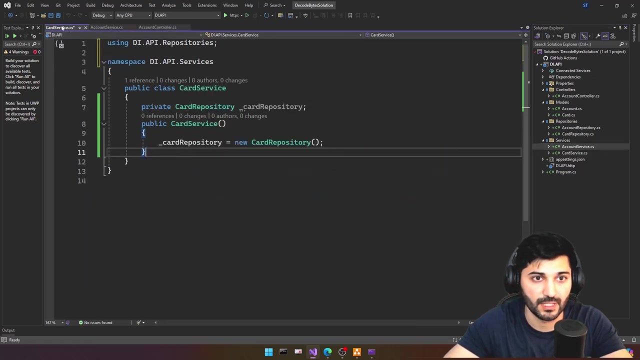 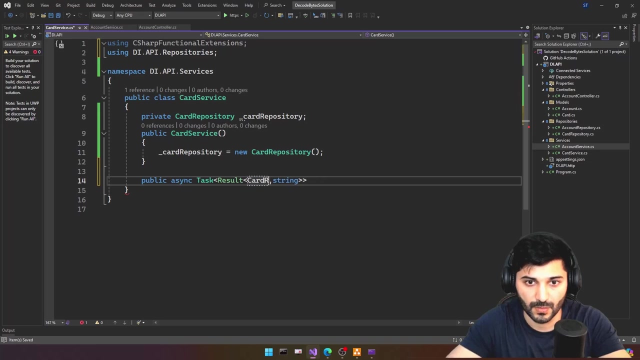 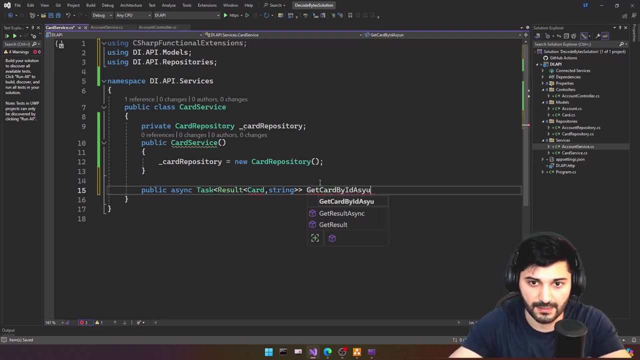 great, let's go to our card service. okay, for the card service, we have card repository, we have instantiated this one and the same approach will follow here. and let me, just from the service, return public async task result. this is our result: card string, card string. okay, let's add: using get card by id asynchronously. 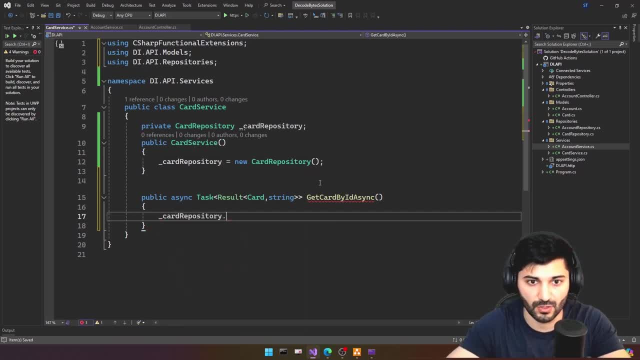 and we'll just delegate this responsibility to our card. okay, get by the id asynchronously. let's provide this um card id and await our card. if card düşüttürürn Clipboard. if card is null, then return result: dot fulfill card. if card is null, return result: dot fulfill. 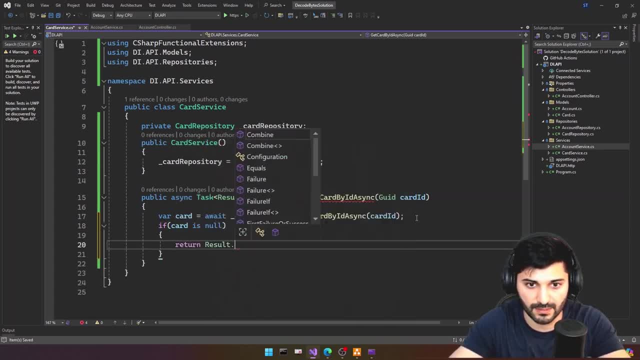 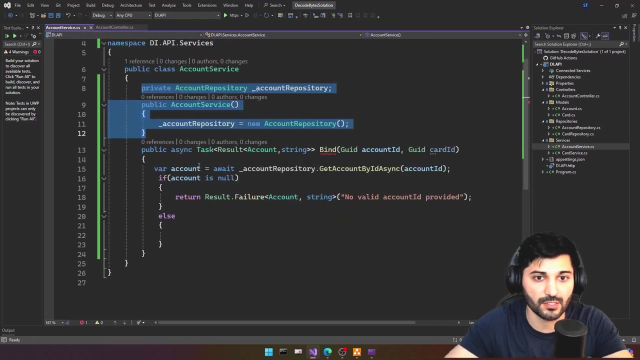 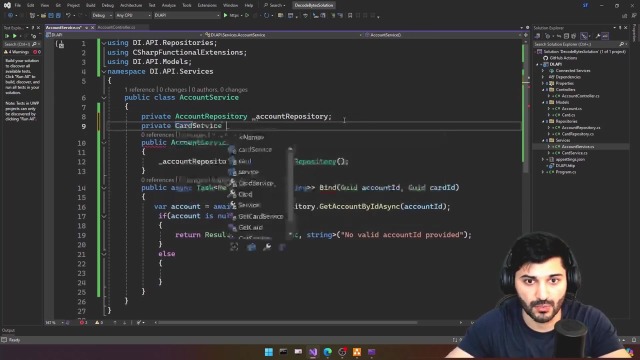 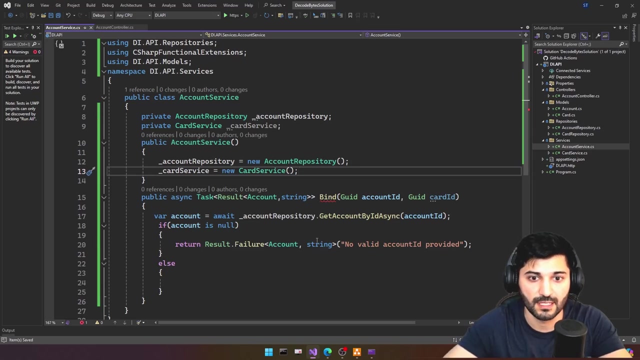 card is null, then return result: dot: fulfill dot failure card string: okay, card string: not a valid card id. otherwise return result: dot: success card information: great, now we have card service. we are able to use our card service here, private card service. this is our card service and let's instantiate it and let's just go and 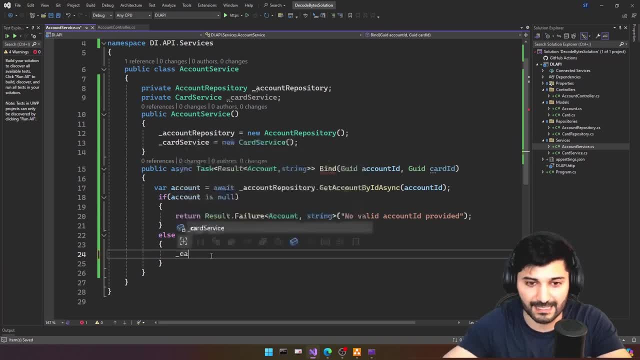 use it. if our account exists, we need to check our card service. get by id. let's provide our card id and this is our awaitable operation: var card- and again, if card is null, then we will return. respond that something is wrong. let's wait for it. this is result. so we need to check. something like this is failure. 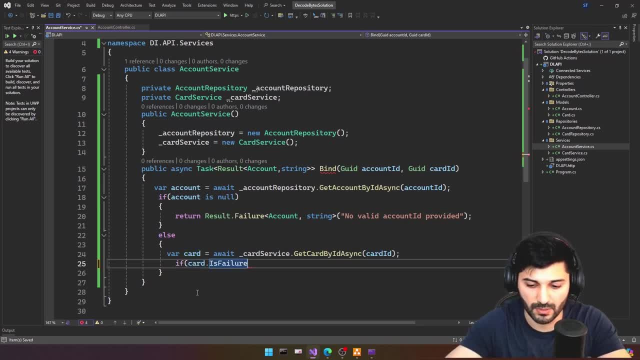 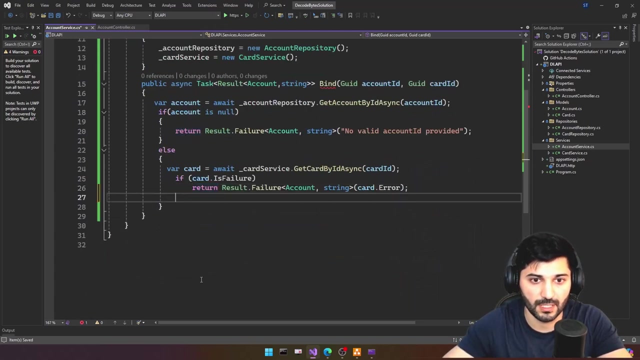 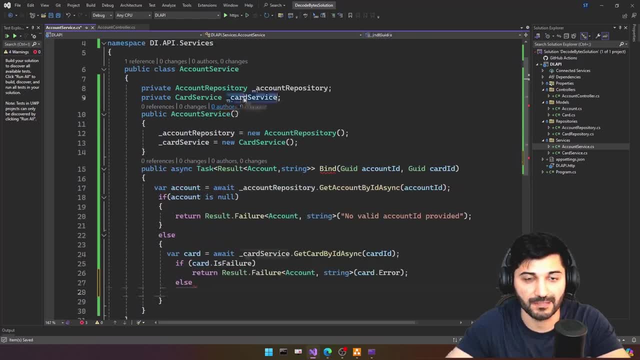 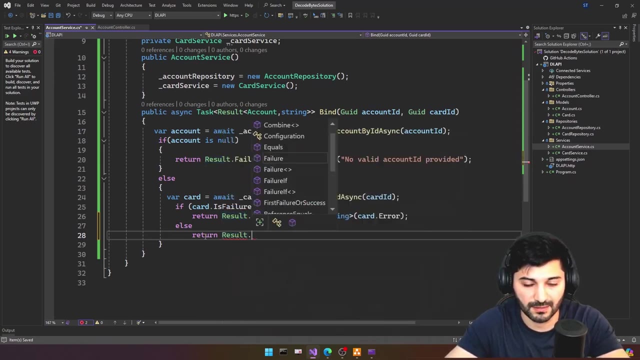 what i'm going to do is i'm going to do. i will have another method here for card service. i will add it to my repository. you can use a unit of work etc. but for simplicity i will just return that return result dot, success account string and let's return our. 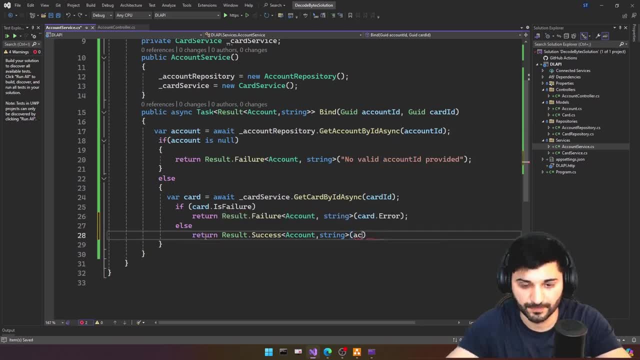 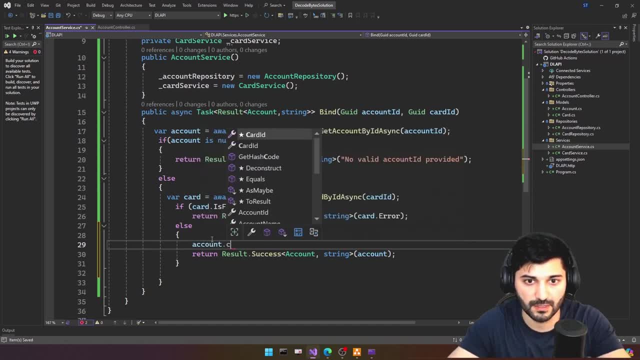 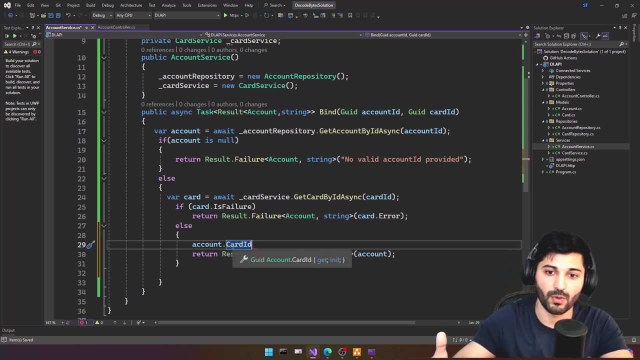 with given card. okay, let's cut paste it here: uh, our account dot card id. uh, our account dot card id. uh, our account dot card id. okay, and for the given card id, i will provide okay. and for the given card id, i will provide okay. and for the given card id, i will provide the responsibility to. 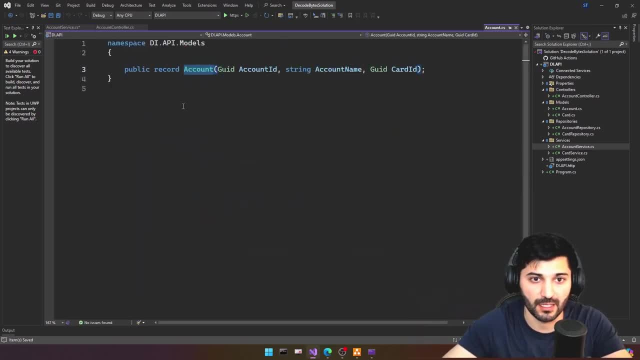 the responsibility, to the responsibility to get this information. so i'm going to my get this information. so i'm going to my get this information, so i'm going to my account, account, account and let's change syntax a little bit. and let's change syntax a little bit. 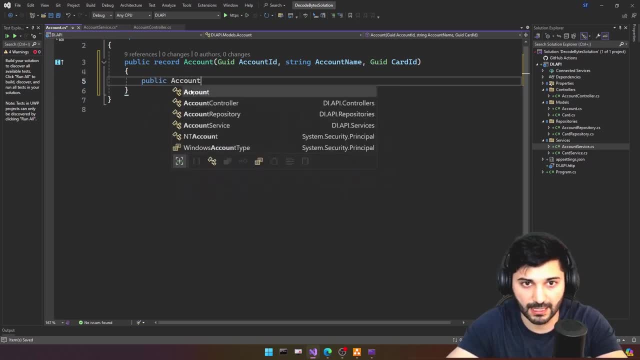 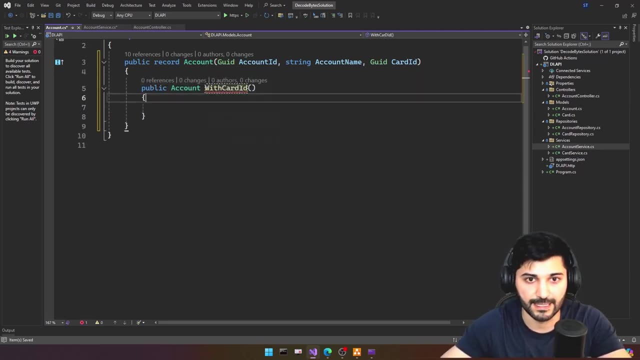 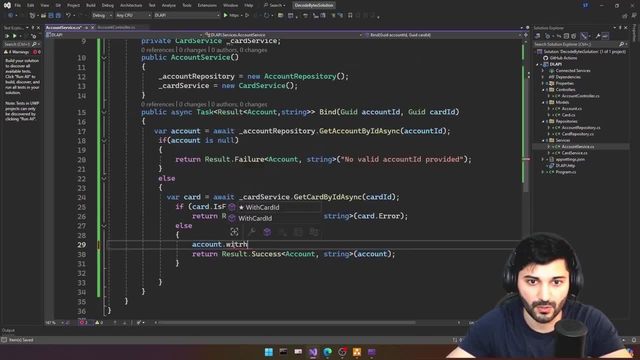 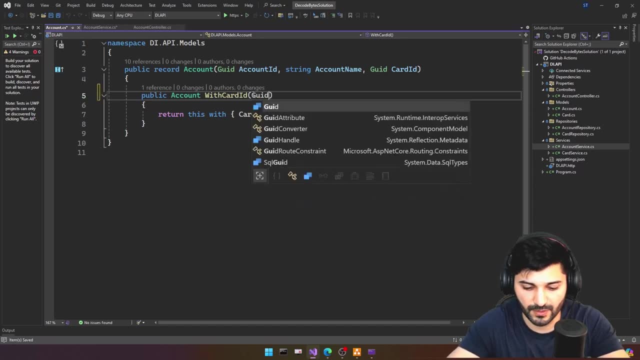 with card id equal to card id. with card id equal to card id. great and account. great and account. great and account. with card id. with card id, with card id, i guess, i guess, i guess, go to definition, go to definition, go to definition and, of course, grid card id. 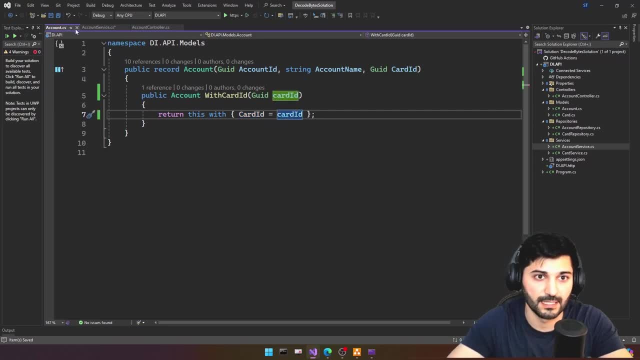 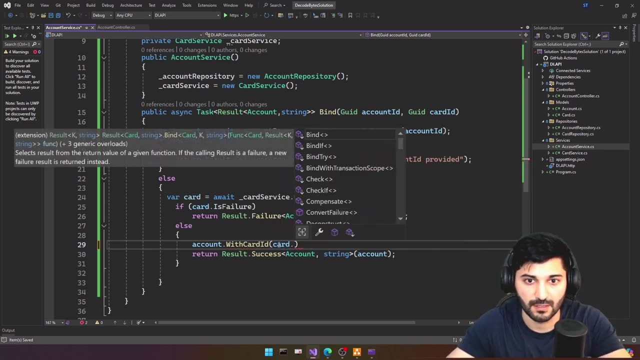 and, of course, grid card id and of course, grid card id will be here, will be here, will be here: card id, card id, and let's provide our, and let's provide our and let's provide our cards, cards, cards id. here is our card. so the result: 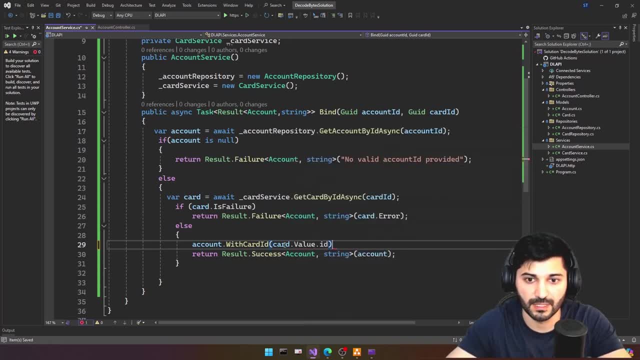 id. here is our card, so the result: id. here is our card, so the result: um, um, um value, not value, not value, not id. or we can use our card id id, or we can use our card id id, or we can use our card id. that's also completely okay. 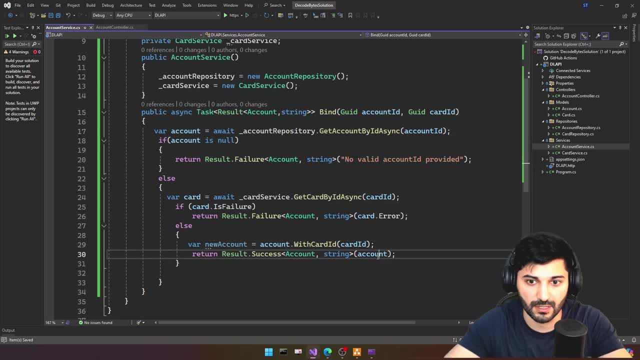 that's also completely okay. that's also completely okay. our new account- let's get our new account, our new account. let's get our new account, our new account. let's get our new account and use our new account and use our new account and use our new account account. 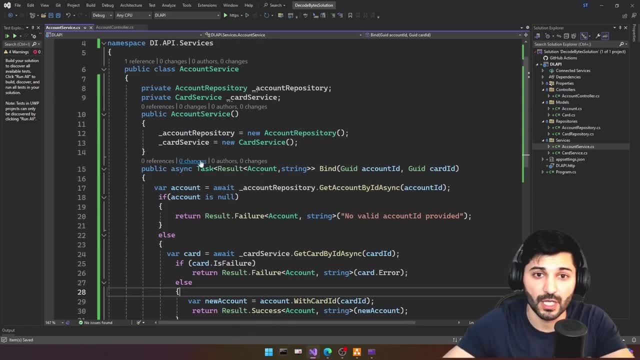 account, account. this is our success case. so what we are, this is our success case. so what we are, this is our success case. so what we are going to do here, we are going to use our going to do here. we are going to use our going to do here. we are going to use our repository, direct repositories. you see, 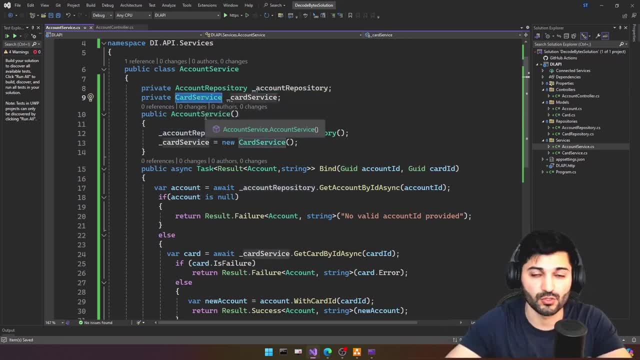 repository direct repositories. you see repository direct repositories. you see, we have card service. here we are, we have card service. here we are, we have card service. here we are directly using card service. we are not directly using card service. we are not directly using card service, we are not using interfaces, etc. 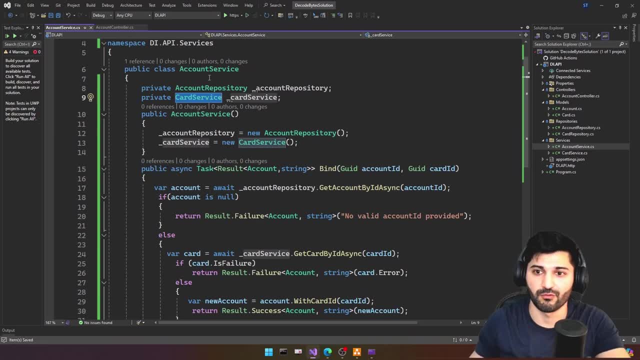 using interfaces etc. using interfaces etc. and uh, this is going to be a little bit and uh, this is going to be a little bit and uh, this is going to be a little bit problematic for us. problematic for us, problematic for us, of course. and here we have the card. 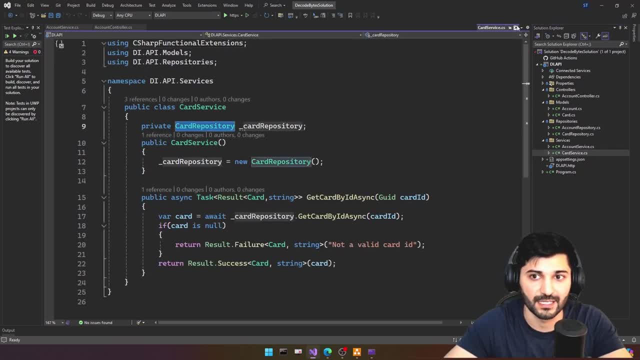 of course, and here we have the card, of course, and here we have the card service which is going to use our card service, which is going to use our card service, which is going to use our card repository, repository, repository, directly, directly, directly. now let's go to our controller here and 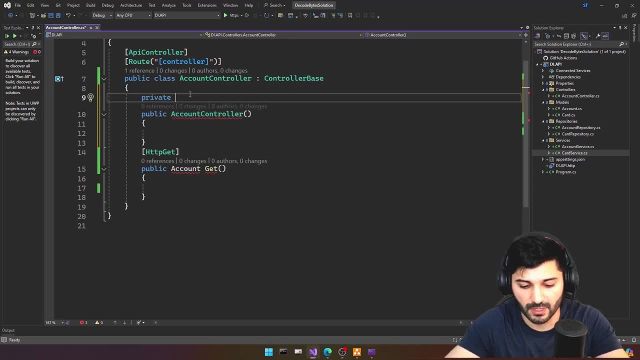 now let's go to our controller here and now let's go to our controller here and let's instantiate our private. let's instantiate our private. let's instantiate our private account service. this is our account account service. this is our account account service. this is our account service. 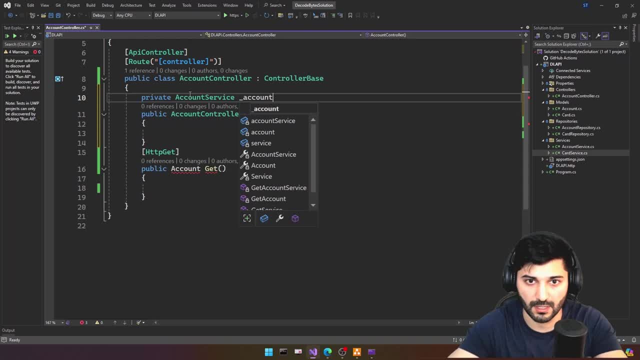 service service: ops, ops, ops. this is our, this is our, this is our account service, account service, account service, and and and for the account service. let's instantiate for the account service, let's instantiate for the account service. let's instantiate this account service, this account service, this account service, and let's use it. 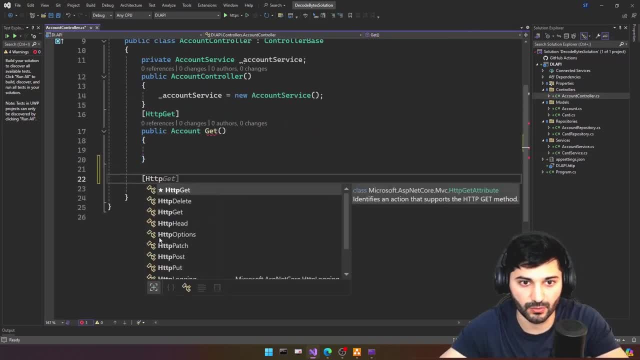 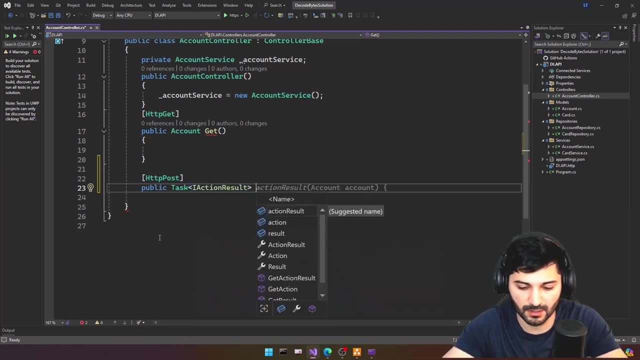 and let's use it. and let's use it. implement our binding process for that. implement our binding process for that, implement our binding process. for that reason, i will use reason. i will use reason. i will use http posture, http posture, http posture. public, public, public task. i action result. 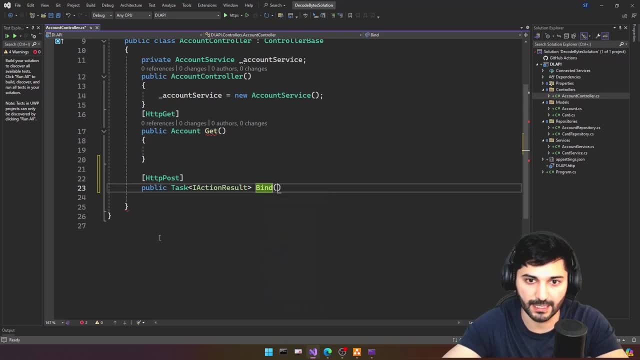 task i- action result. task i- action result. let's call it buy and simply buy, and i let's call it buy and simply buy, and i let's call it buy and simply buy and i will use, will use, will use grid account id and give it our. 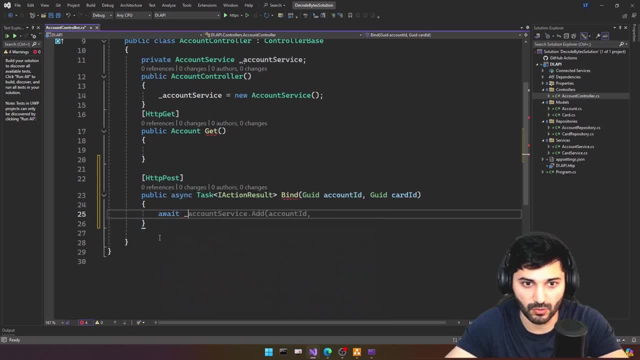 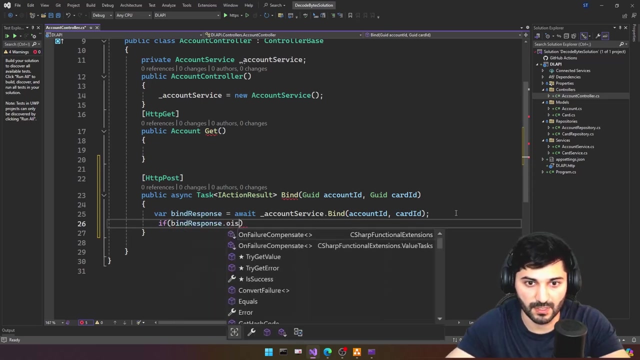 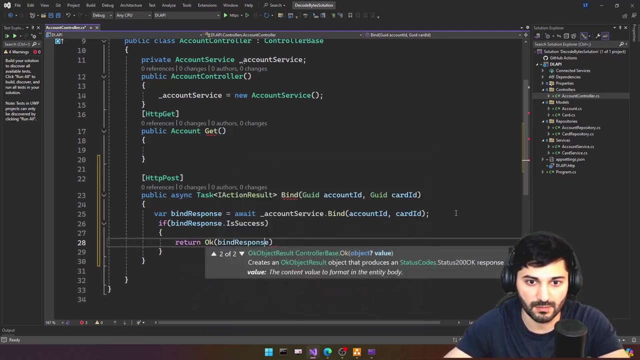 grid account id and give it our grid account id and give it our card id, card id card id: okay, and let's call our available: okay, and let's call our available: okay, and let's call our available not, not, not, okay, with bind responsevalue. okay, with bind responsevalue otherwise. 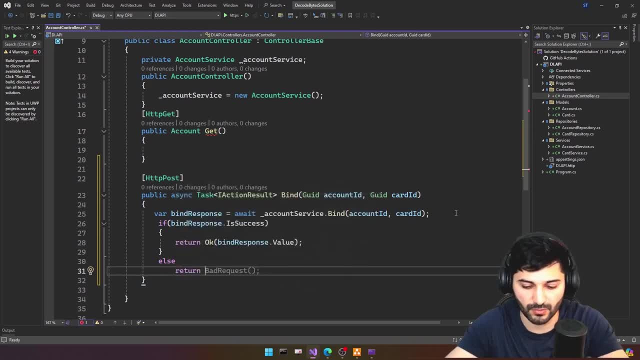 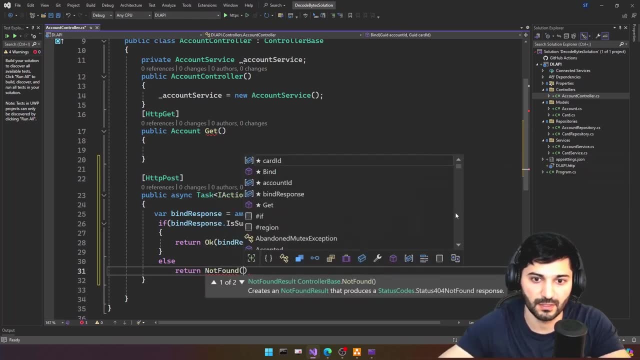 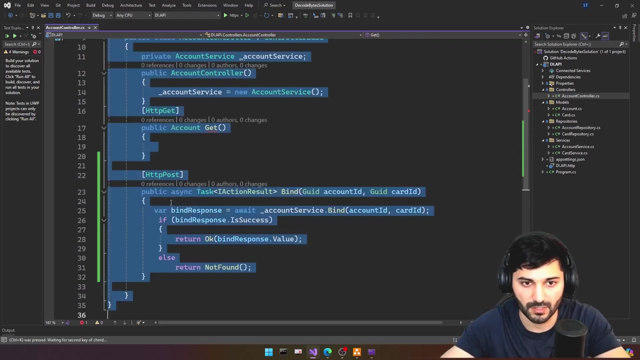 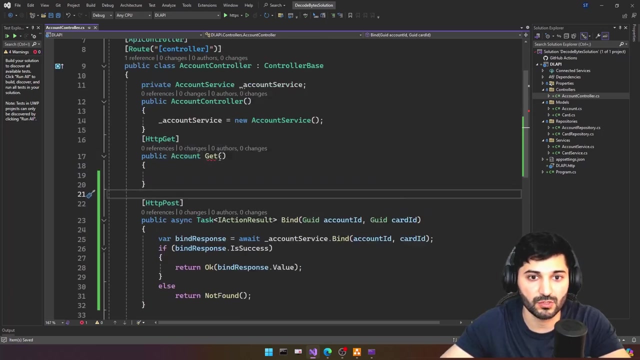 otherwise it means something is wrong. let's return. i don't know, not found, maybe not found, i guess. so let's see the loading version. i guess that should be okay. let's just i'm not going to provide the error message or etc. for the simplicity. that should be okay. and from the accounts service. 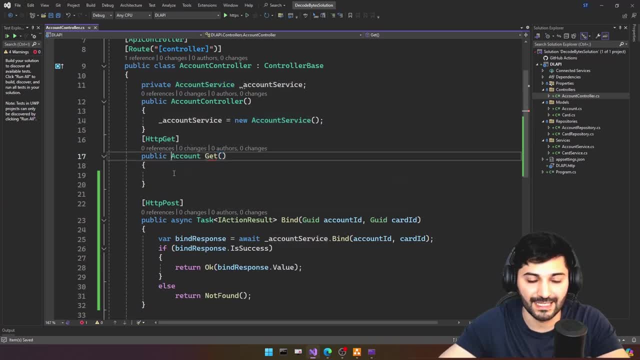 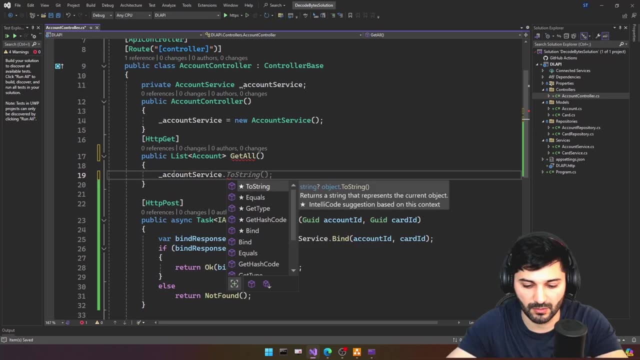 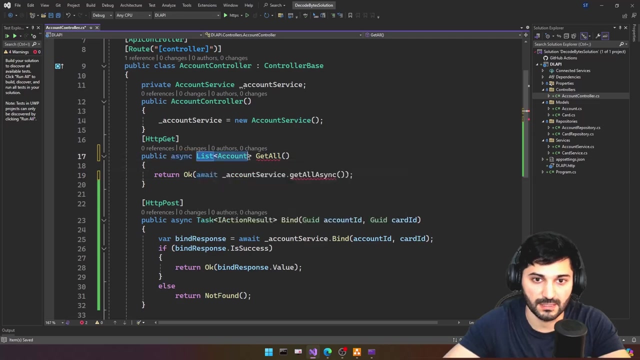 i will use to return all data: public list, account get all and i will just use account service get all and, of course, async and awaitable return. okay, great, i guess. for the return, okay, we will just simply use task i action results. great, let's just implement this method. 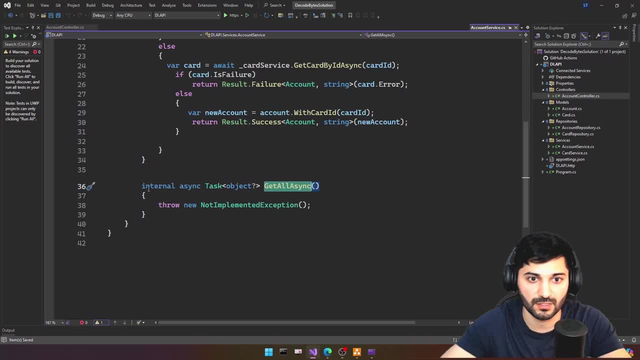 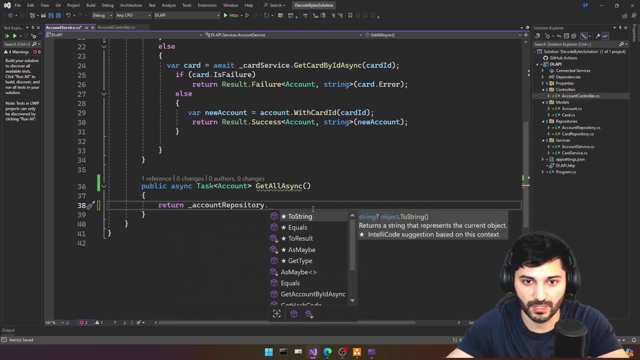 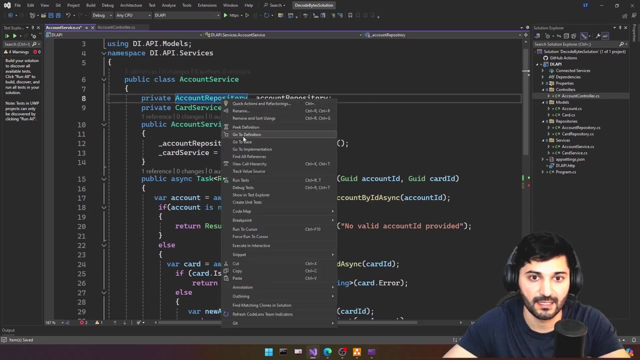 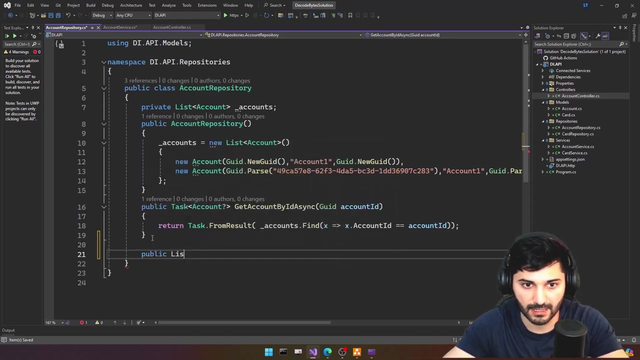 generate this method. go to definition, public task account and let's return return account repository dot for the account repository we have. we should have get all type of syncs. go to definition and public list account or a enumerable account, it doesn't matter. get accounts, get accounts. 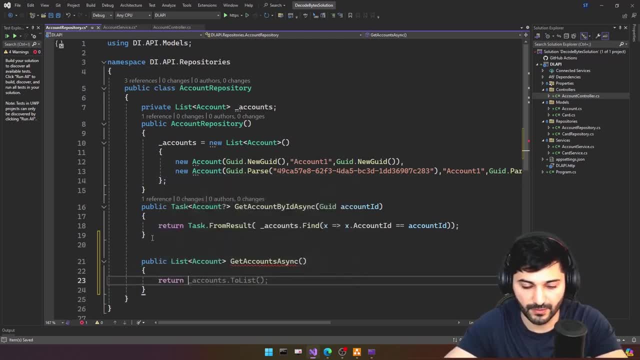 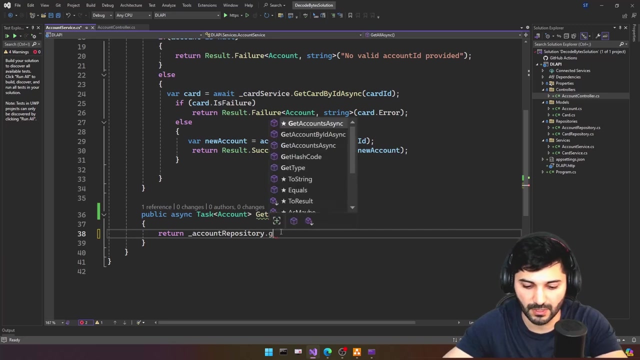 asynchronously return task. that from result, accounts dot. i think just accounts okay. so let's see list: accounts okay, task from result, task list, great. and let's go to our account: get all. get all accounts asynchronously and waitable. yes, we just need to make at least account, get all. 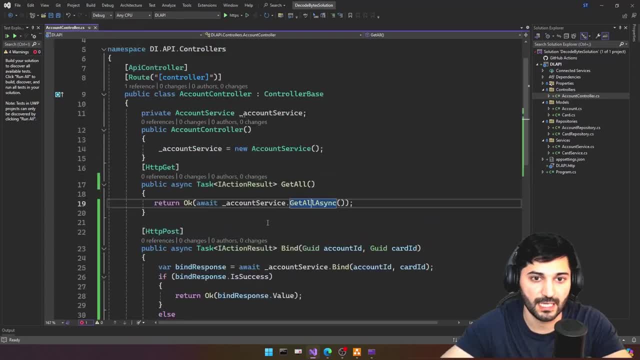 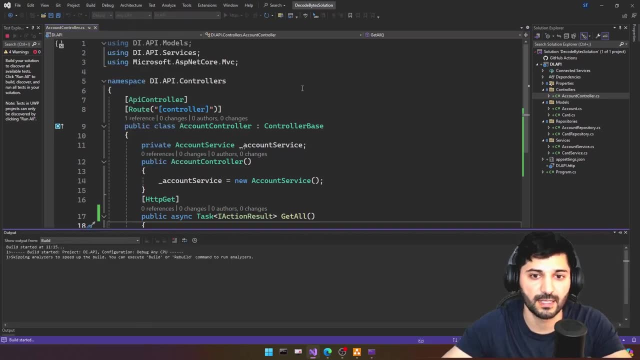 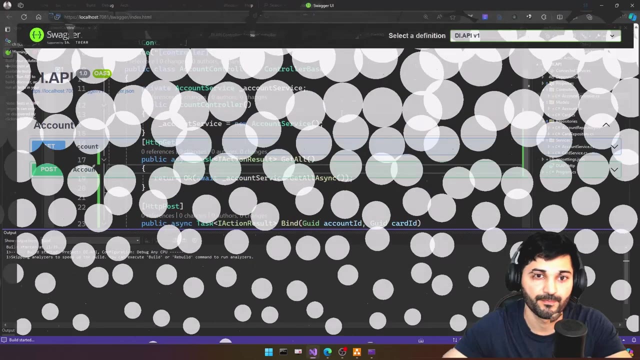 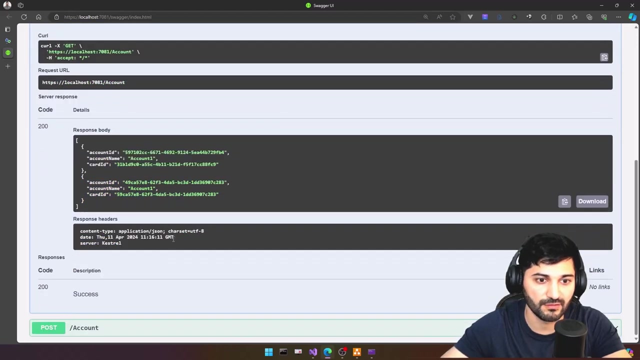 account, get all, get all asynchronously and let's go and check if everything is working. debug, start without debugging, and let's see we should have two endpoints: one for get and the second one for post. great, now we have get, let's go for it, let's execute. and here we are. we have all this account information to make the 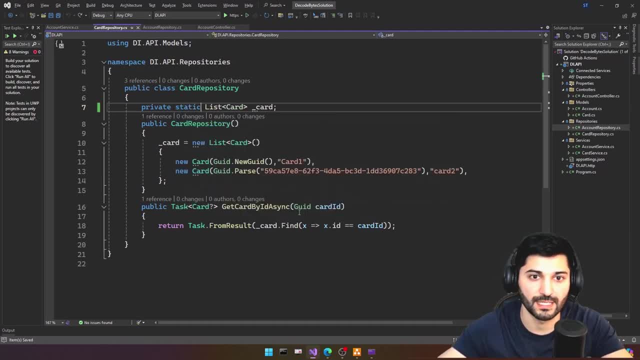 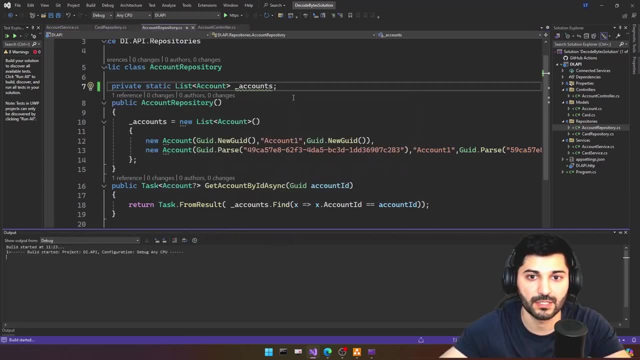 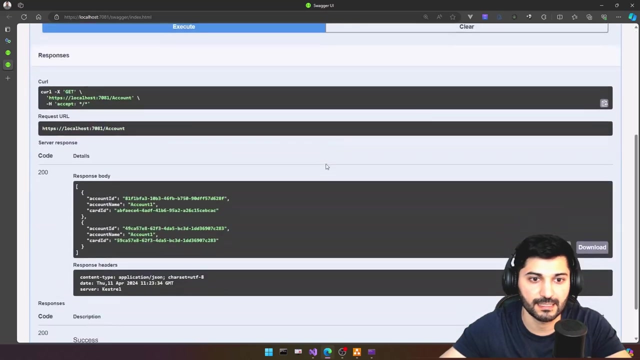 list to not to refresh every request. we need to provide a static. here. let's go to our account. also, let's provide our static data and let's debug our application again. and here we are. let's go to our get, let's execute. so you see, this is eight one, but nine, four, nine. 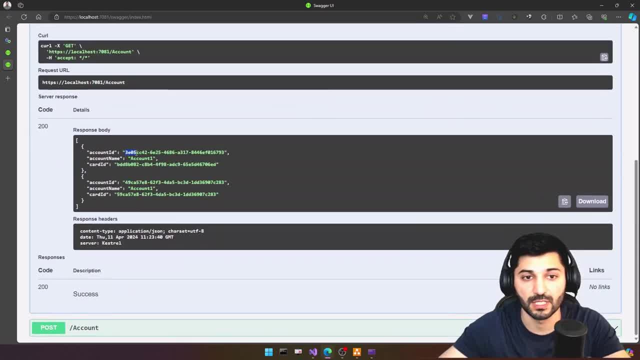 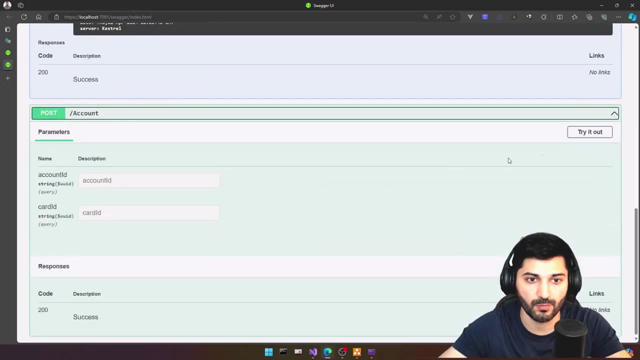 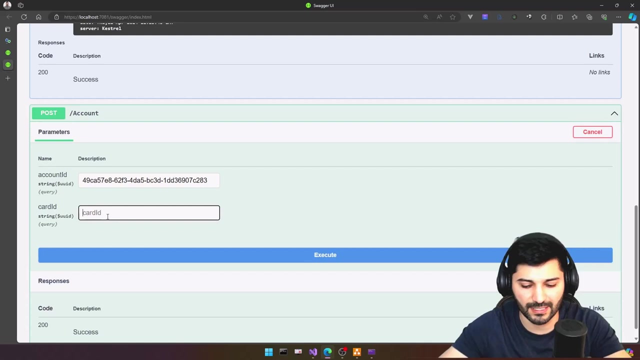 let's execute the four nine states, but this will be different value because we have give it that new account id here. so what i'm going to do, i'm just going to copy this information from here, okay, and let's go to our account post, let's provide our account and i'm going to use the exact cart id. right now, we 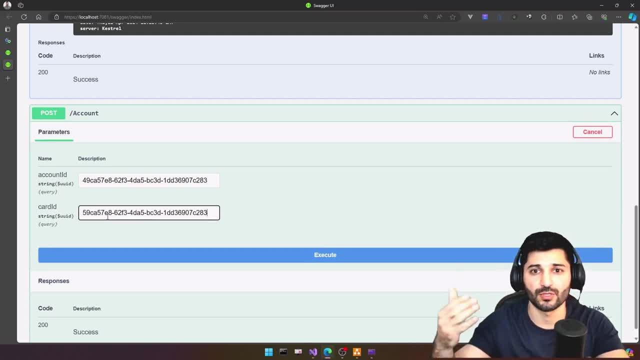 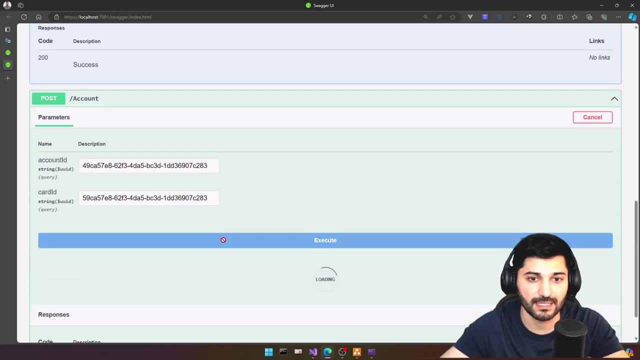 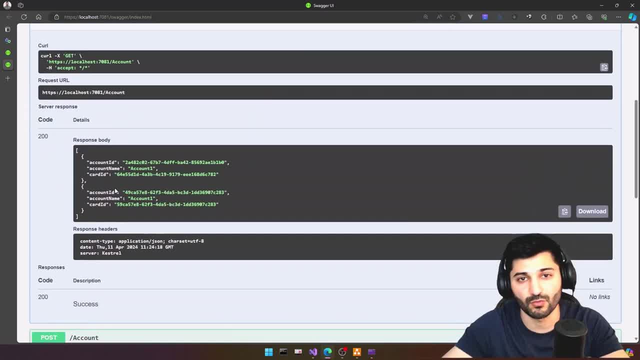 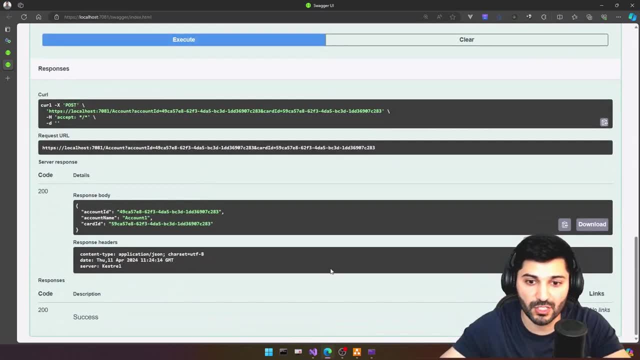 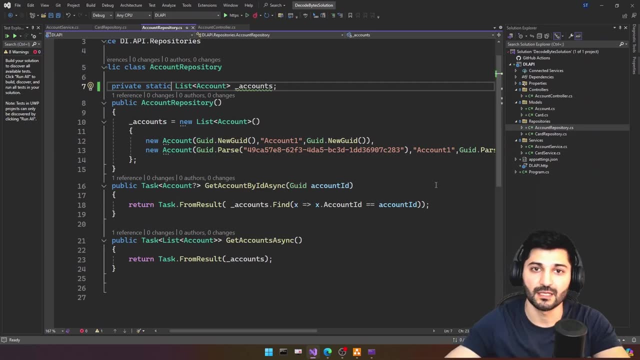 is working and let's execute. now we have two values again because we haven't added to our repository, but that's completely okay. we are getting the success information and that's all how. we are simply implementing all this stuff, of course. uh, this is not a bit um, correct application. 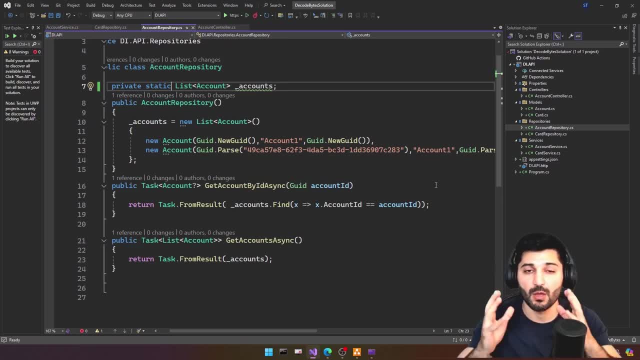 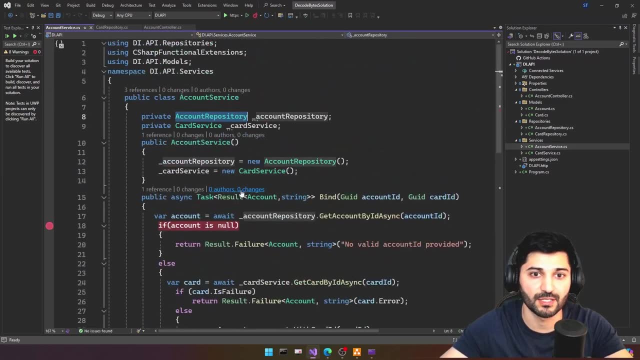 to use. the purpose here is to show that we have multiple dependencies in our classes. for example, let's go for our account service. in our account service we have dependencies in our classes and we have dependencies from our account repository and card repository. and when you go to card, 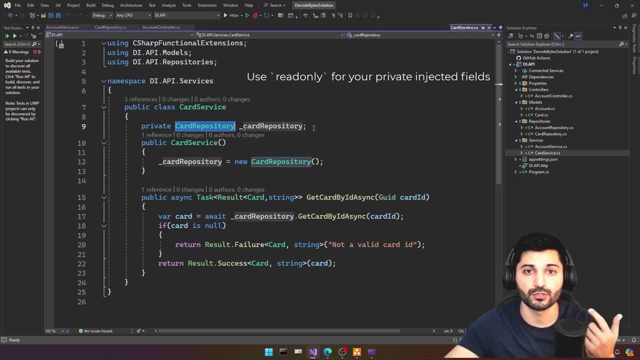 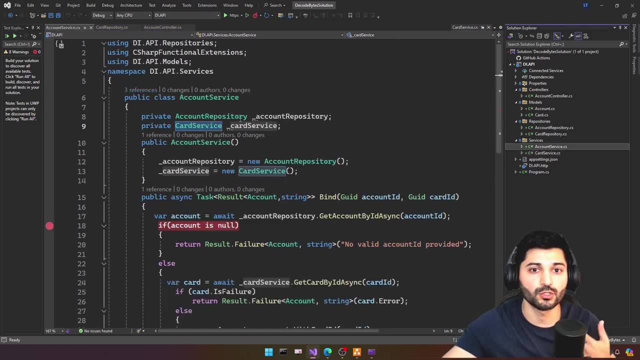 repository. it has dependency from card. when you go to card service, you have dependency from card repository. of course, that's completely okay, but what if i want to change my repository? so what is the problem? the problem here is i may have multiple implementation of my repository. i 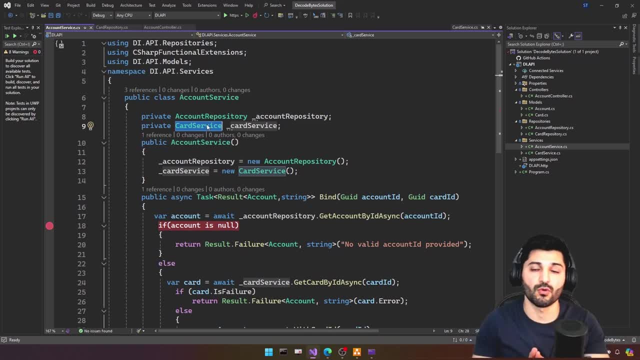 may have especially multiple implementation of my card service, but right now my application directly depends from account repository and it is internally implemented, this card service also, the account repository also. this is a big problem for us because if you want to test your class it will be really problematic because in your application if you want to stop it. 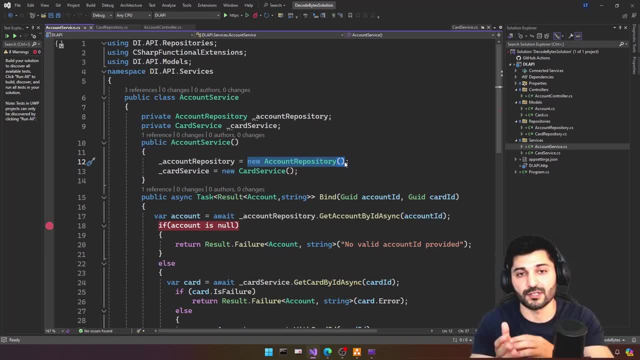 to mockify it. you will just directly instantiate the real data, and it will be a huge problem for us. so what should we do now? we are going to test our class and we are going to test our class we do here. of course, it is better to provide it from the arguments, but if you provide it from the 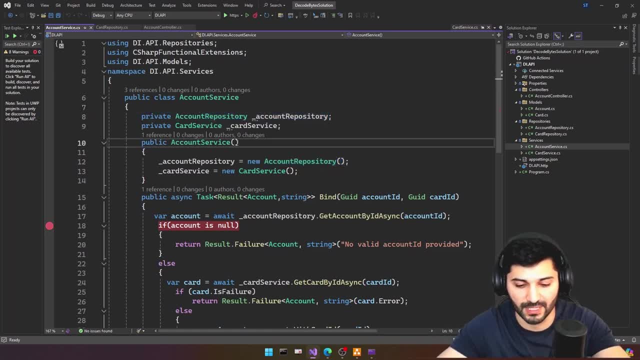 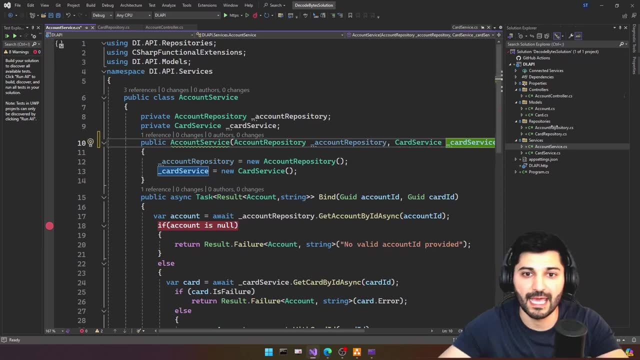 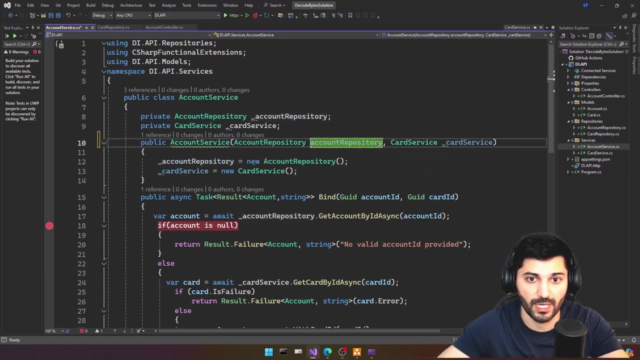 arguments. you have again direct dependency from the implementation. let's say, i'm providing this information here like this, but still i have direct dependency. okay, so i'm providing this account information here, so let's provide it. i'm not going to instantiate any stuff here. okay, this is my account repository. and for the card service, let's, for the card service, use our. 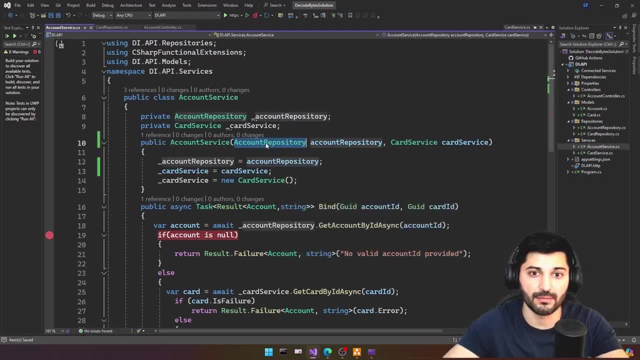 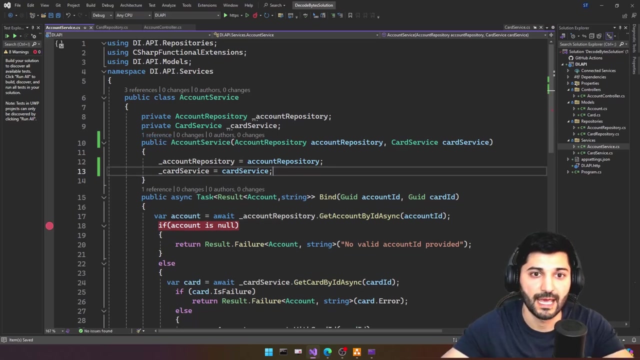 card service. now it is a little bit okay because it is possible for you to make this uh repo or these services, some functionalities- virtual, to override it in your testing process, but still you have direct dependency from account repository and card repository. let me just remove this one from here and let's see in this case, as you might guess, when you are constructing, 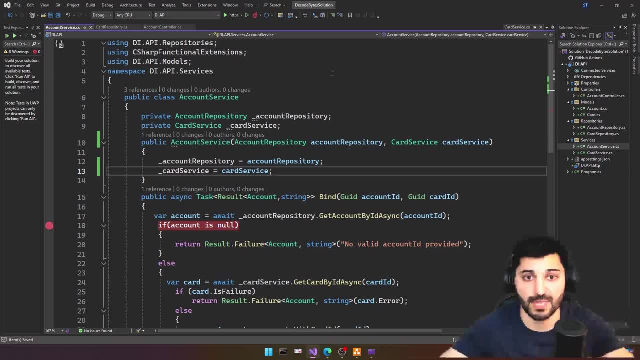 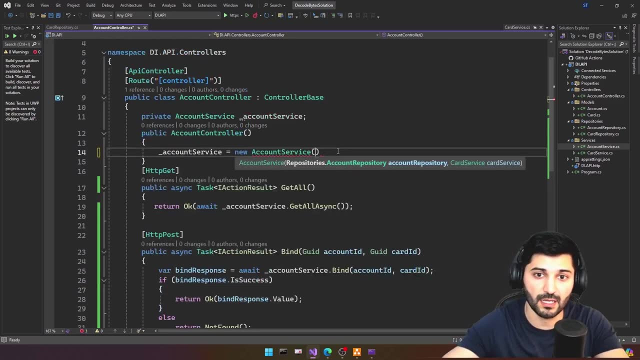 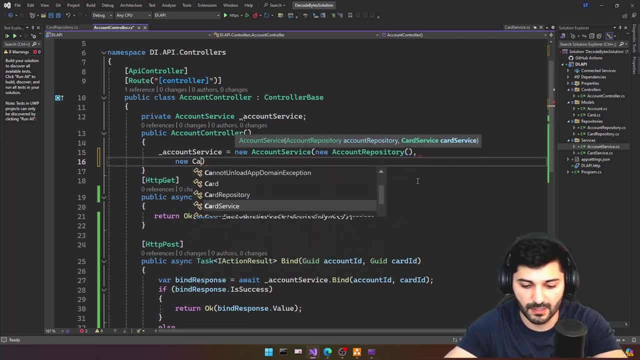 some class. you may have multiple dependencies, especially in our account service. what i want to do? i want to instantiate my account service, but my account service will require account repository. let's instantiate this account repository here. account repository, account repository- okay. and the second dependency is card service. let's check this card service, but this card service. 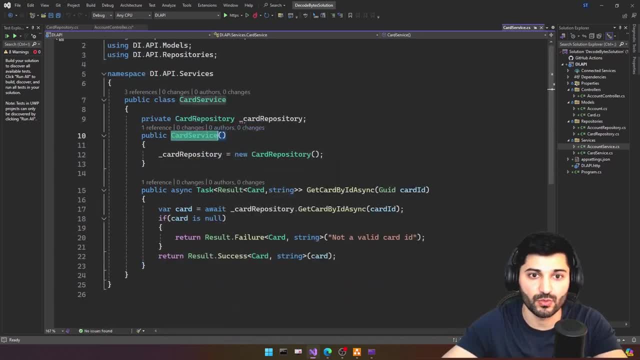 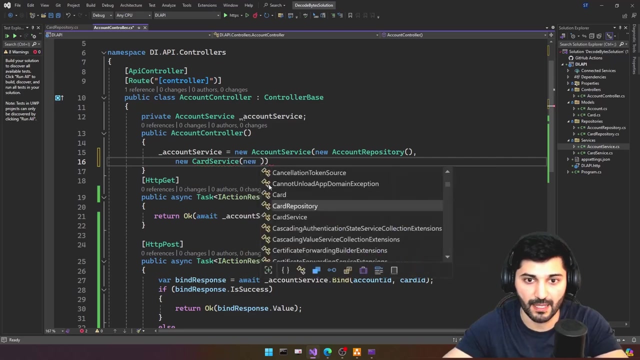 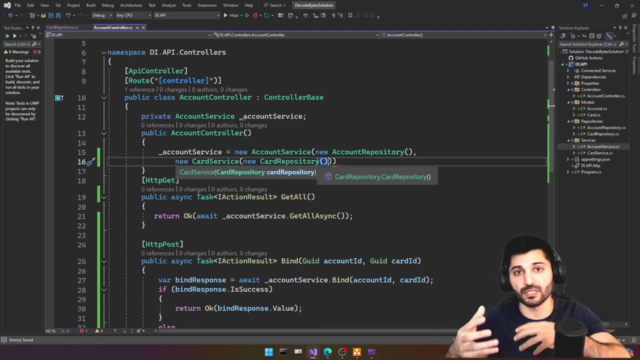 also may have some dependency which we are going to inject right now. this is our dependency here. now i am not going to construct it internally, but for uh provided from my constructor, okay, the card repository, of course. now, here you see, i have another dependency, so this dependency also may have another dependency and this will be, uh, a big problem for you to 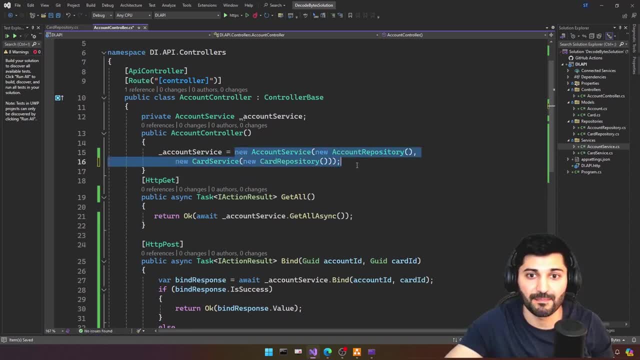 construct your object. you see now it is a bit complex. my account service requires a counterparty and on the other hand it requires card service, which card service requires card repository. So you see, you have all the knowledge here directly in your controller, and every time when you use account service or some sort of complex service like account service, you will provide all the implementation manually in your code by your own. 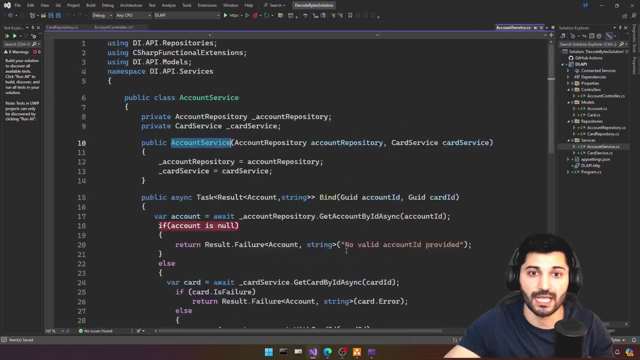 This is a big problem And also, as I mentioned, another big problem is we have: the main problem here is we have direct dependency from the implementations. For example, account service uses card service. What if I have a strategy based card service? I mean, for example, right now I'm using this card service, but I will need another, completely different implementation of card service. 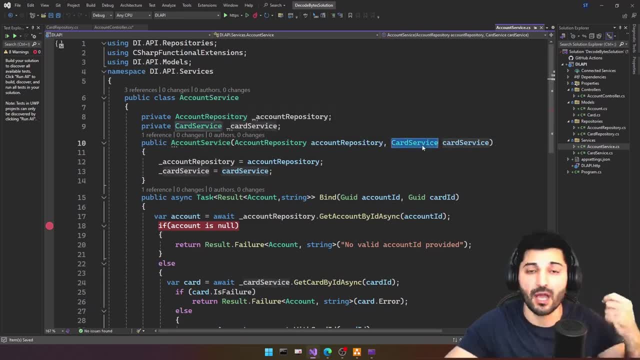 But my account service directly requires card service. So we need to somehow abstract out from this card service here. So it means you should provide abstract class or interface here to isolate your application from direct dependencies. This is the real purpose behind dependency injection. Okay, now let's talk about dependency injection. 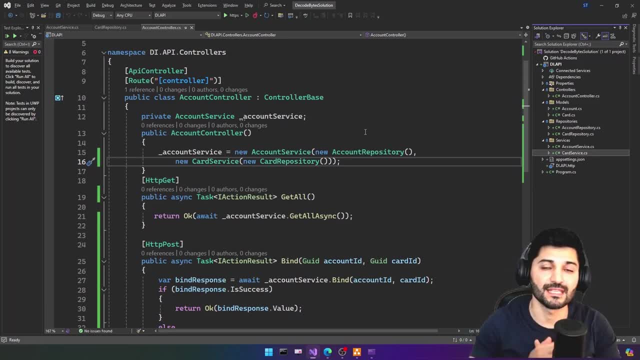 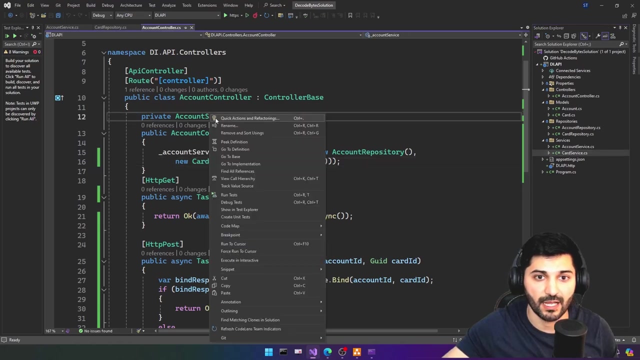 Dependency injection is an implementation form of dependency inversion principle, which we are going to talk about in our next tutorials. This is also a big topic. This is one of the principles of solid. The last D is dependency inversion. Dependency inversion means that your high level modules shouldn't depend from your low level modules. Both should depend from abstraction. In my case, I have account service here and this account service has dependencies from a counterpoint. 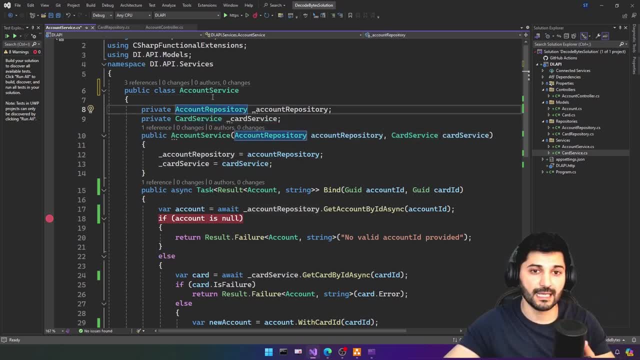 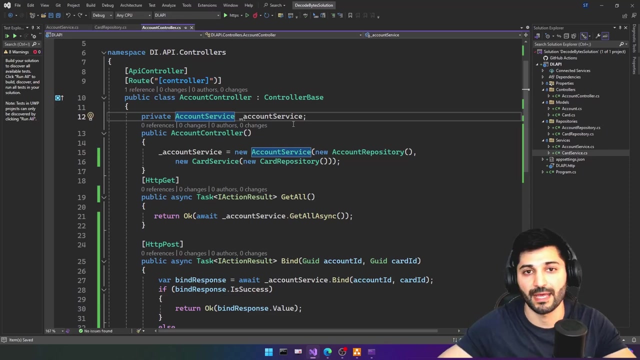 And in this case this is high level module, This is low level module And I have direct dependency from a counterpoint or a low level module depends from a high level module depends from low level module, But it is better to have a communication, like both should depend from abstraction And it means in our controller we need to do some additional refactoring And how we can implement it. let's switch to our applications. 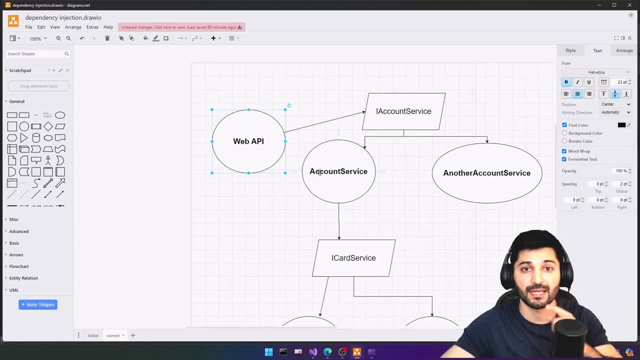 Here we have web API. Now our web API doesn't depend from account service. It simply depends from my account service. Okay, This is special interface that will help us to inject to use any implementation of this interface. It means I can, in runtime, to change my account service to another account service or any other account service that implements I account service. So instead of having direct dependency from this implementation, we can implement it in our account service. 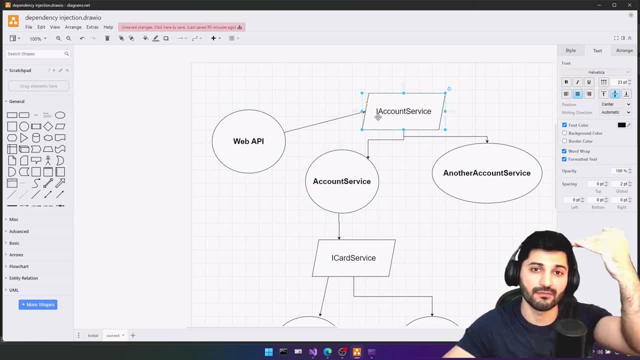 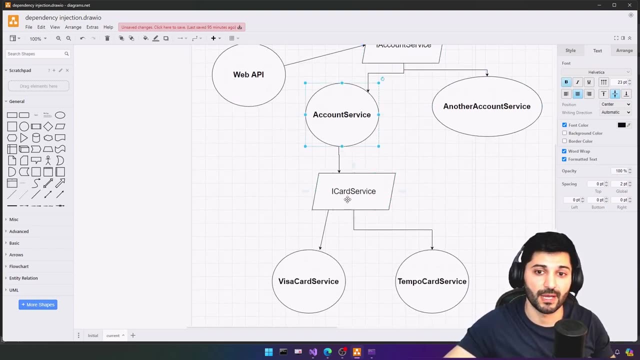 implementation. i have dependency from high level stuff and using this high level interface, i am able to inject the implementation, the exact implementation i want to have for my application. the same is applicable for account service. also, in my account service, i don't have dependency. in our case, we have something like this: yeah, so this is our just simple card service and in this case, 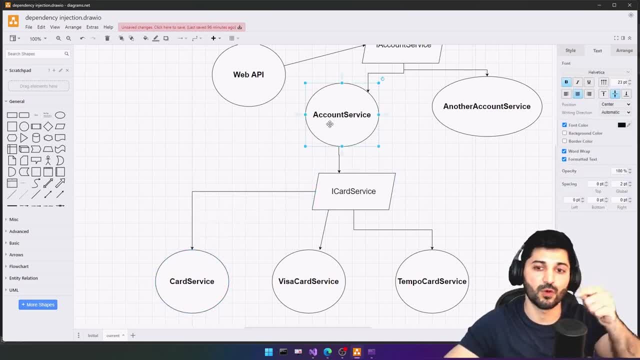 we have direct dependency from card service. our account service uses card service, but when your account service depends from iCard service, it means you are able to provide any implementation of this interface. it might be the card service, visa card service, tempo card service, etc. so it provides us to have reusability, maintainability, extensibility, testability, because in our case, 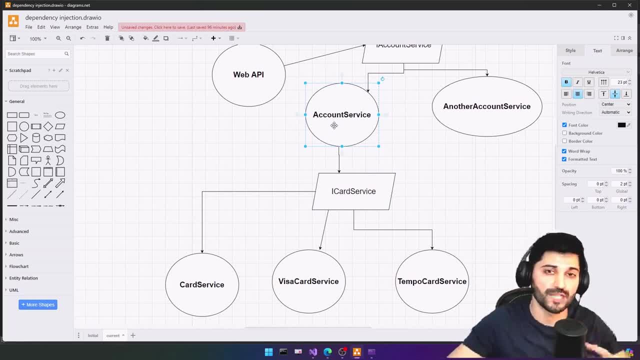 when we want to isolate our account service and to test it. it will not be possible because in our account service we have direct dependency from repository. it is not possible to unit test it if you are not configuring it to provide some virtual methods etc. and this is a big problem for us. it is better to have 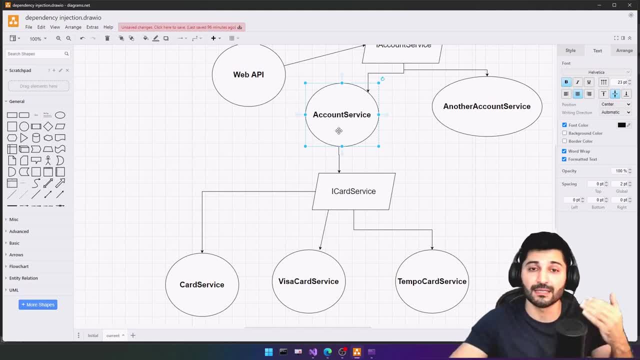 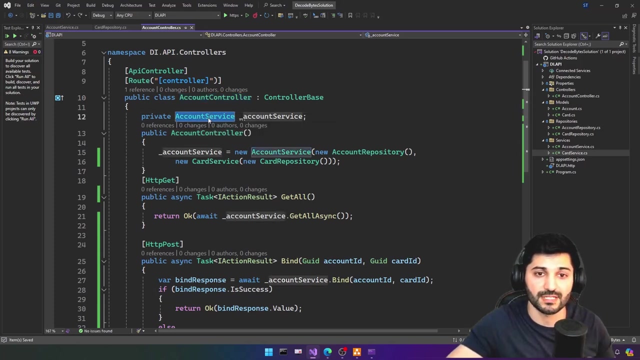 dependency from the interface and to easily mockify it, stubify it okay. so you see, dependency injection is really helpful mechanism for us to inject the exact dependencies, to help our layer to be work in isolated manner, to be tested in isolated manner. for example, right now, our web API, for example, our account controller knows about account service and this account. 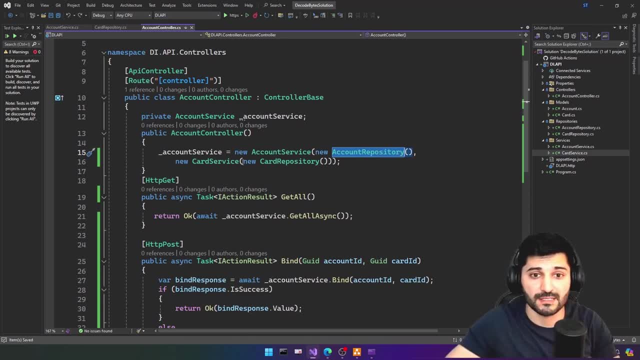 service brings another dependencies like repository, card service, card repository. so you see, we have all the detailed mechanisms here. so this is a big problem for us. we need to isolate our account controller to use, to not depend from the interface. see that we have our anybody device and if you see, 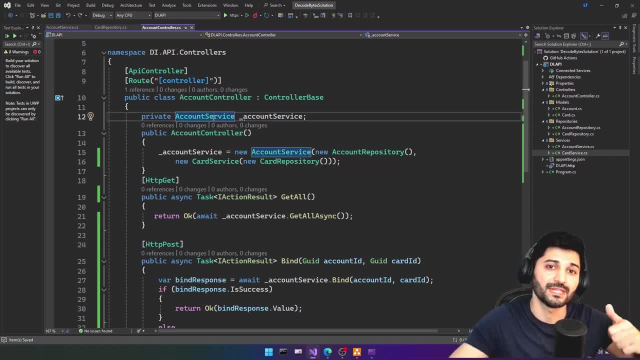 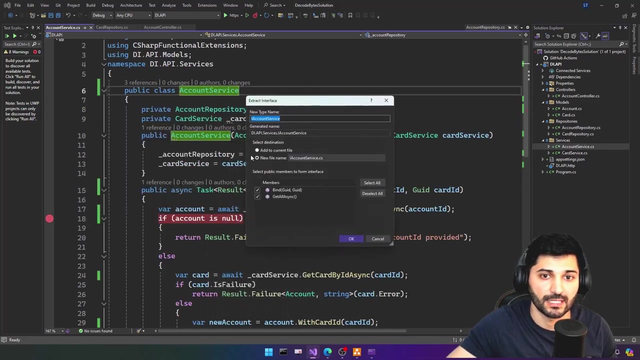 account service implementation but depend from the exact interface of it. so let's refactor it, right click quick actions and let's- uh, just simply, i guess, uh, here we need to go to our account service and right click quick actions and here extract interfaces and let's extract our 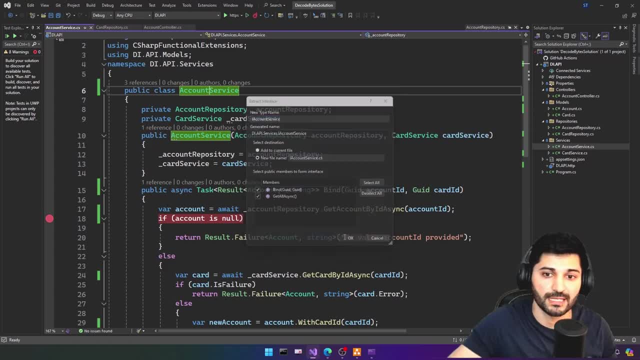 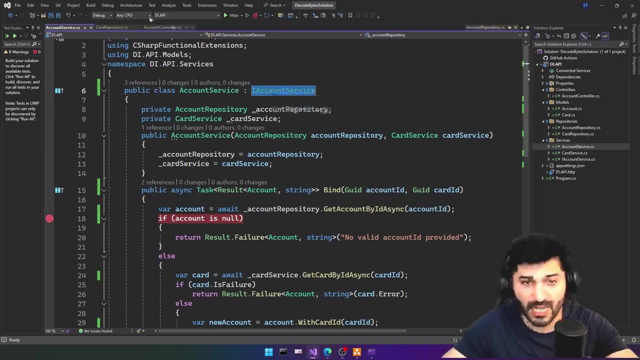 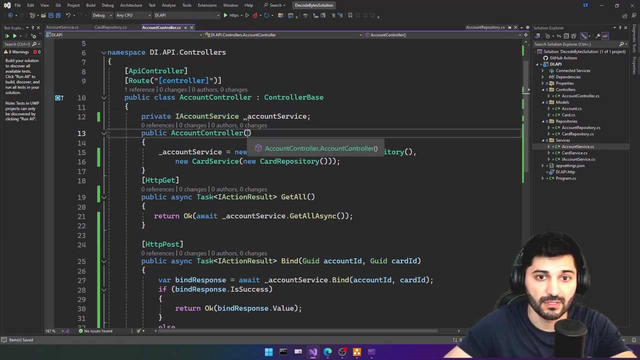 i account service interface. so you see, we have bind, get all. that's great. and now our account service, um implements i account service. i just want to go to my controller and provide that. i'm using i account service and i will provide this account service from constructor to isolate my 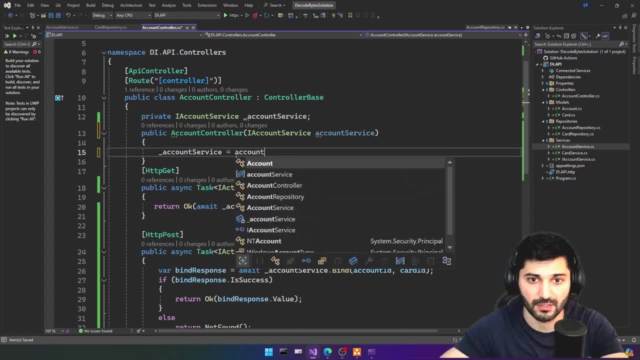 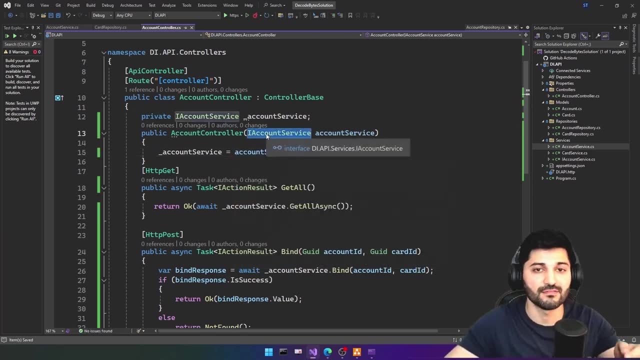 application to this: implementation details: okay, account service, account service, account service- great. now we have dependency from, not to exact implementation, but from i account service. so you see, we don't have any implementation details like the account service that uses the repository stuff, that uses card service. we have completely isolated our application from these dependencies and now 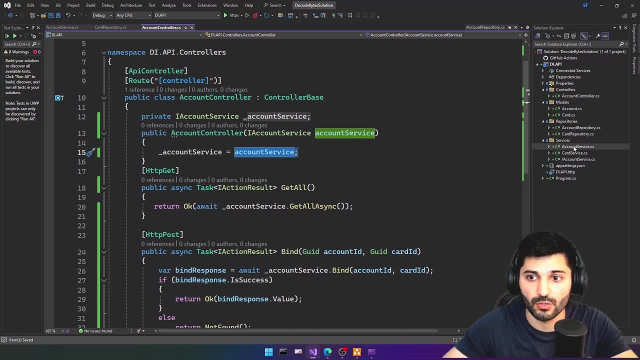 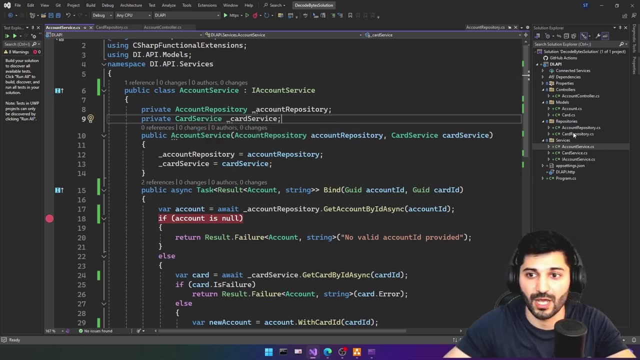 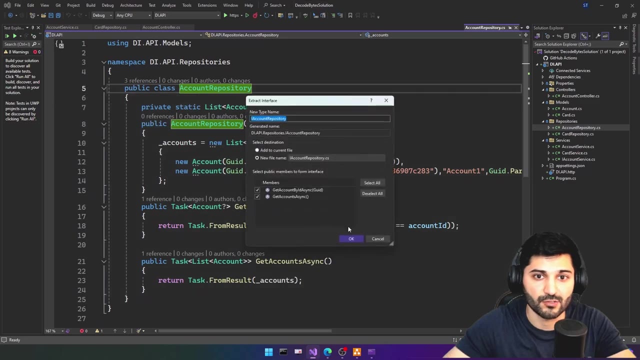 let's go to our card service. of course, our account service of course requires i account repository card service, so we need to isolate them. also. let's go to our account repository, right click, quick actions, extract. i'm creating the same stuff for this account repository. let's follow the 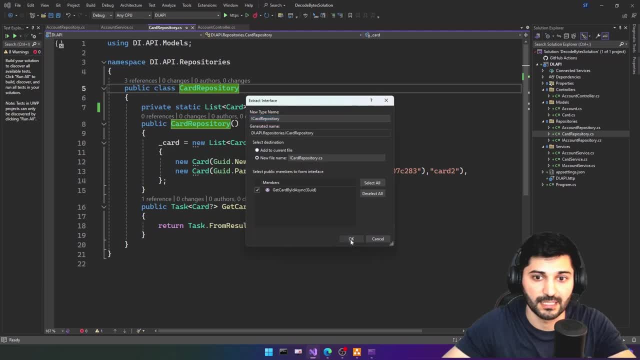 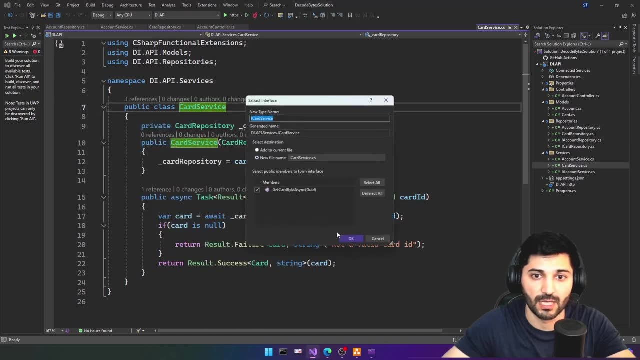 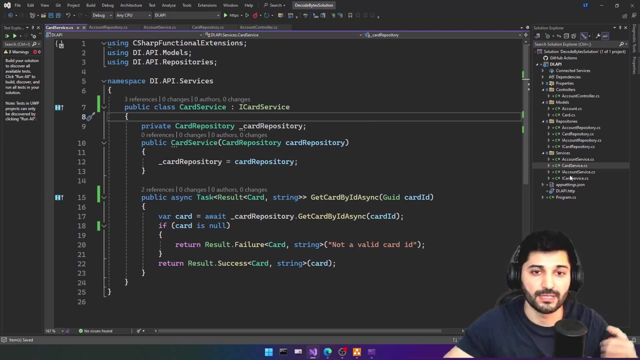 same mechanism here for card. let's create our interface and let's go to our card service and let's create our interface here. so you see, per class, right now we have an interface, interface and it means right now my application will not depend from any implementation low. 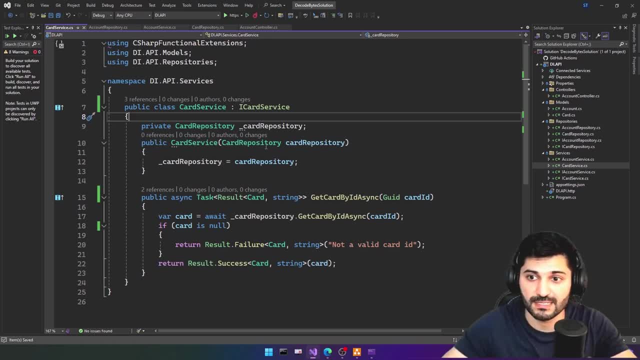 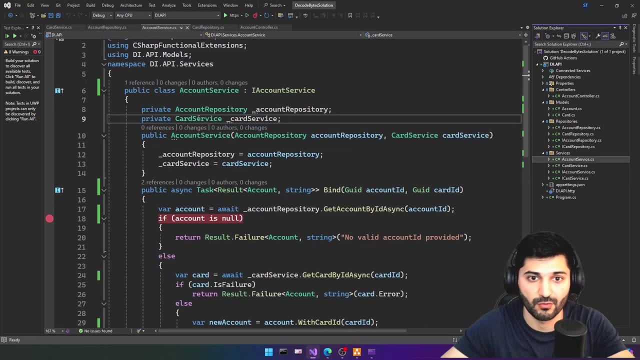 level details. let's go for card service and let's isolate our mechanism here. okay, this is going to be icard repository and from the constructor i will provide icard repository. the same is applicable for account service. i will provide i account service, icard service and from the 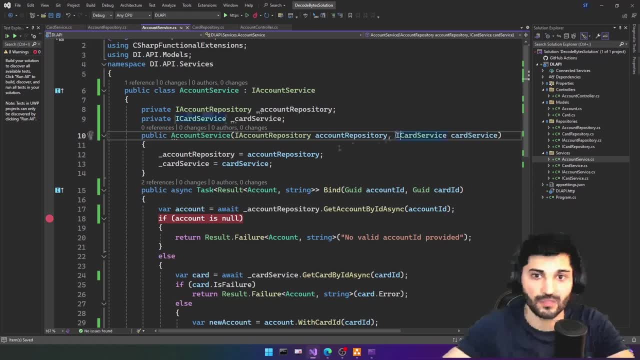 interface, i account and icard service. it is possible to implement dependence injection using different mechanisms: constructor injection, method injection, property injection. we'll talk about it. this is also another big, interesting topic, but for now the popular one is injecting stuff from the constructor. so from the constructor, we are providing these interfaces and you may. 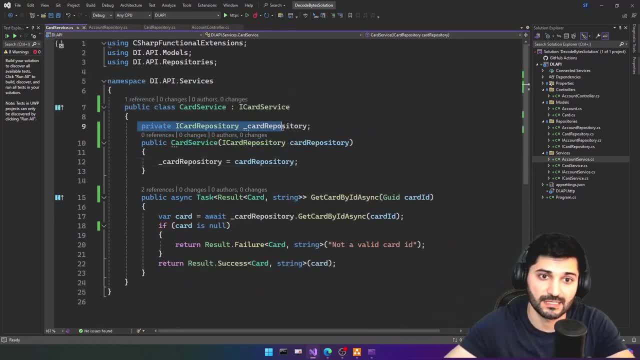 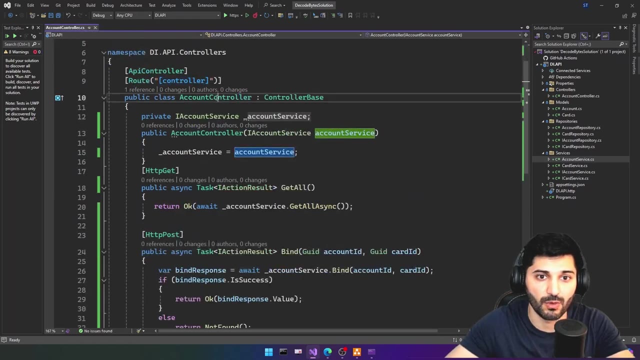 think that, okay, we have implemented this stuff, which seems really cool, but how well, provide this interface to cart service? because we are not using the cart service itself, but we're using this interface. So it is also really easy. Let's go for our account controller. So you see. 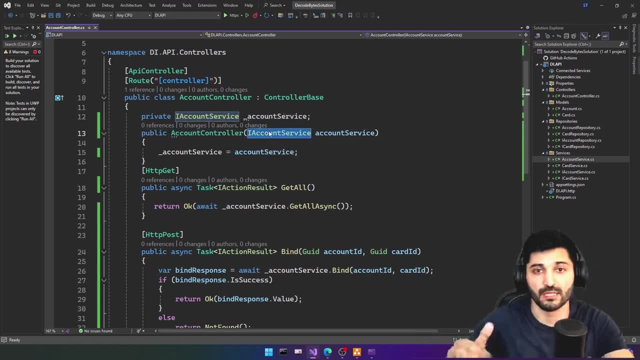 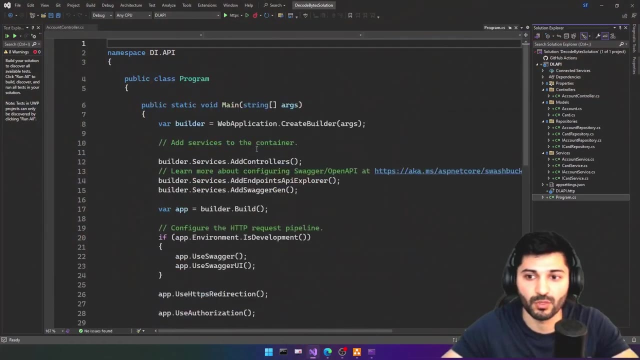 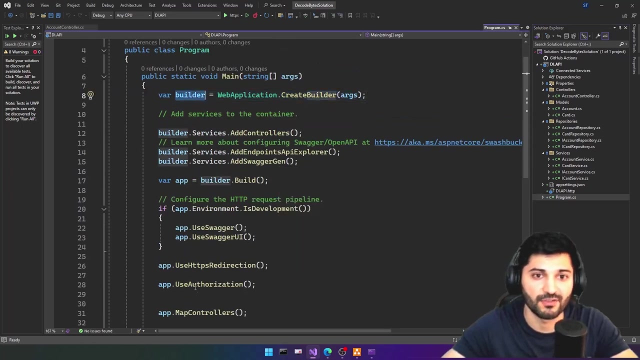 in our account controller we have our account service. This should implement. we will use account service implementation, which is going to use account repository and cart service, And let's configure all these dependencies together To configure dependency injection. we have program cs here. okay, In our program cs we have the building process. we have builder here and we 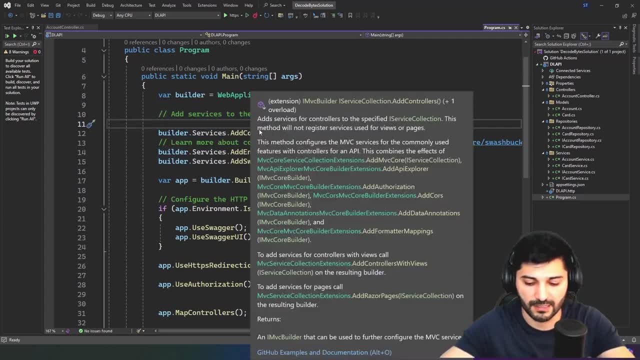 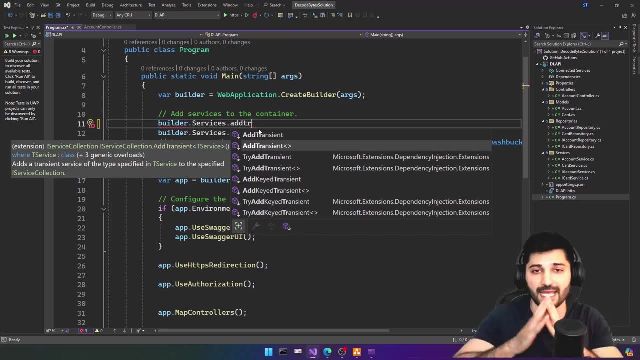 have services. So you see, add services to the container. It means I will provide builder services at transient. We'll talk about at transient right now. This at transient will help us for every request to create a new instance. This is similar like to add scoped, but in add scoped in one request. 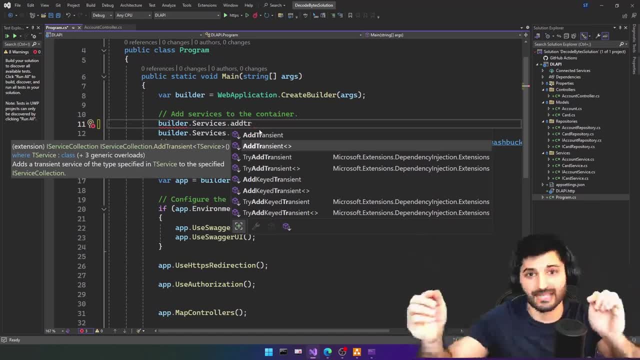 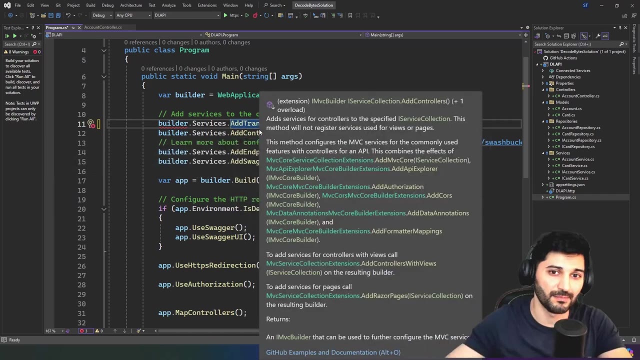 lifecycle for the different classes. if you have the same implementation, if you have same interface system will provide the same instance, But for at transient it will provide every time a new instance of your object. This is not a big problem for us. We are not concentrating to at. 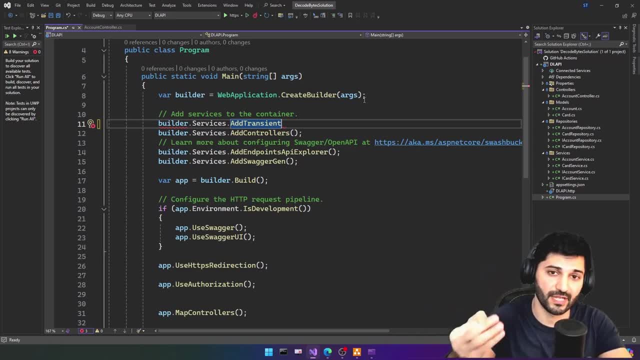 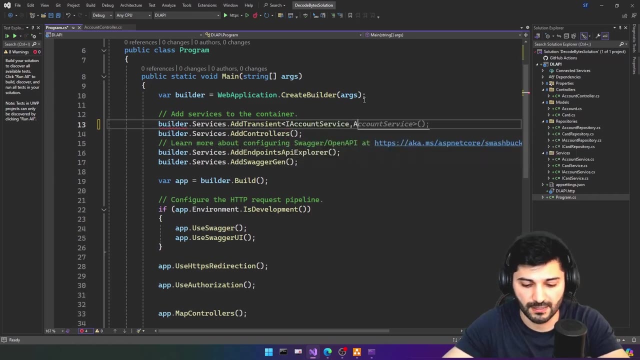 transient at scoped at singleton. We have three ways of injecting these dependencies. Right now let's just try to focus to inject it about lifetime. We'll have another sessions. okay, I'm just going to use account service, Account service. So it means when you see account service, try to create an instance of account. 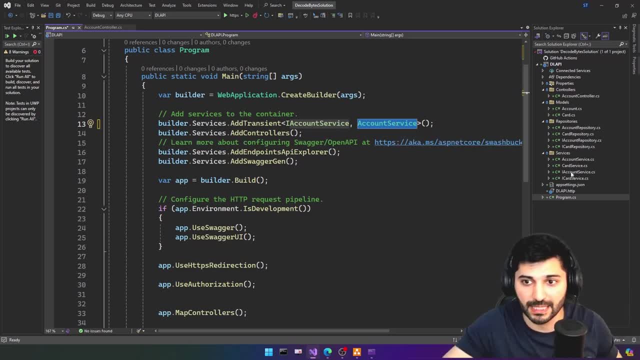 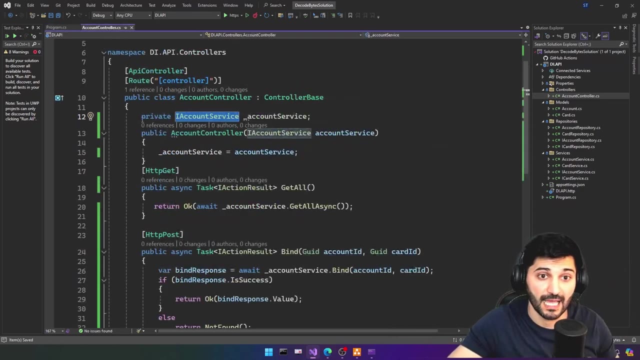 service. okay, And when we run our application, in our application you see we have an account service interface And when you run it, we have build independency injection container and it will monitor our controllers, 볼 clase- and it will check. okay, we have injection here. 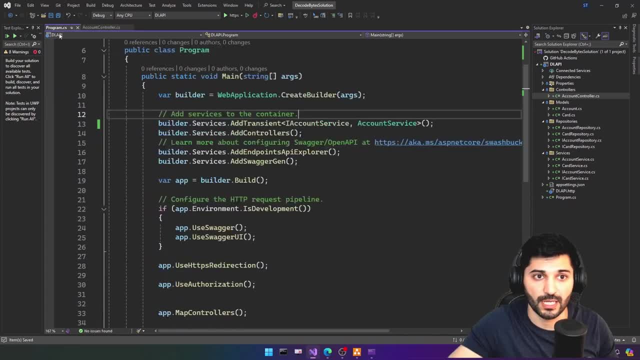 we need to provide a action service. okay, it will check this list and we'll see that we have account service. It means when you see our account service interface, when someone requires account service interface interface, when someone requires account service, when someone has accounts. 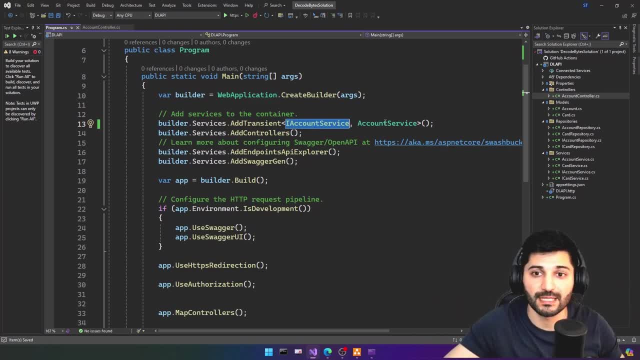 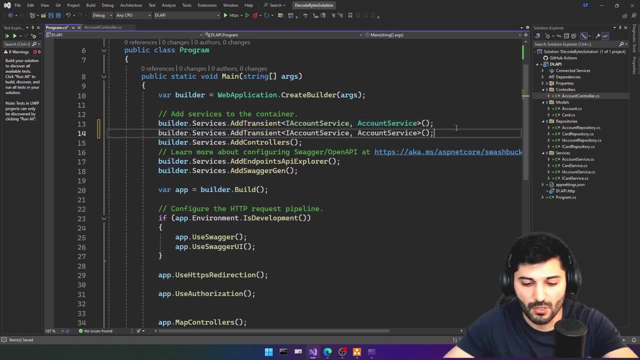 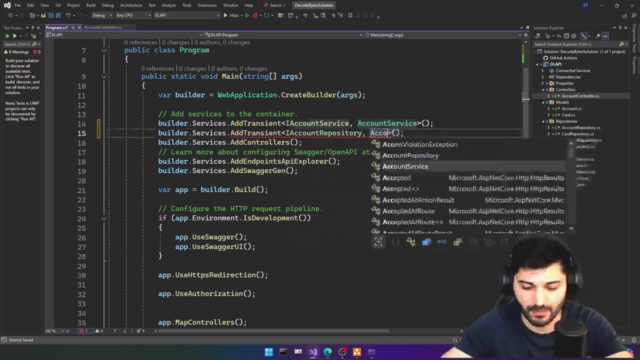 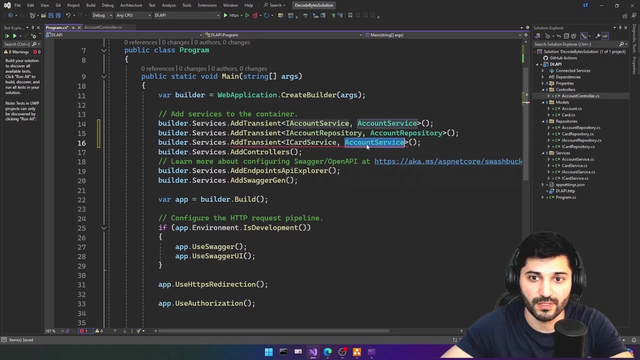 Account. iAccountService provide exact implementation of account service. And let's just copy: For our account service, we need to provide account repository. When you see account repository, provide account repository, And when you see iCardService, provide card service class. 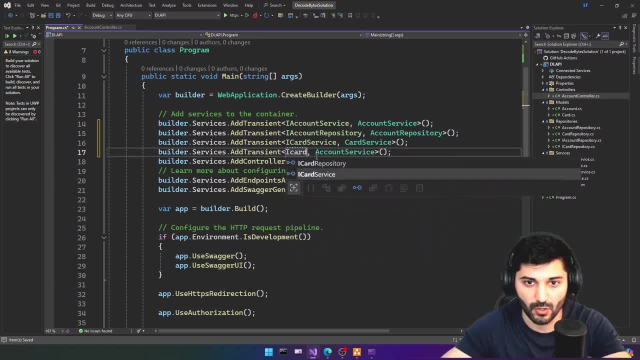 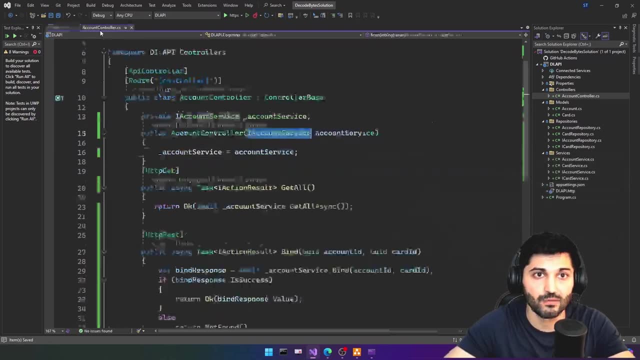 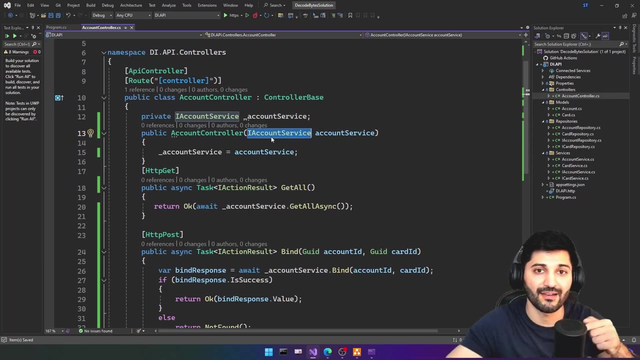 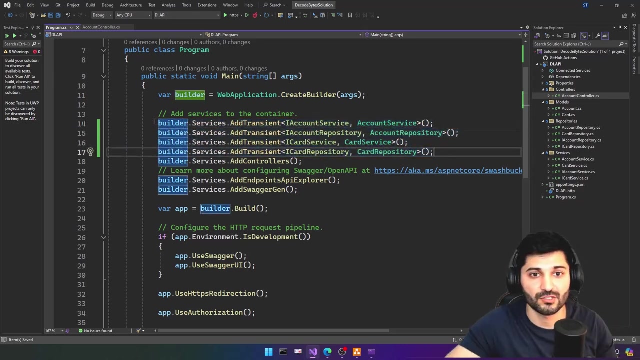 And when you see iCardRepository, provide card repository here. Okay, so it means when we are calling our account controller, it will check if we have dependency or not And if we have exact dependency configuration in our container or not. We are configuring our dependency injection using builder services. 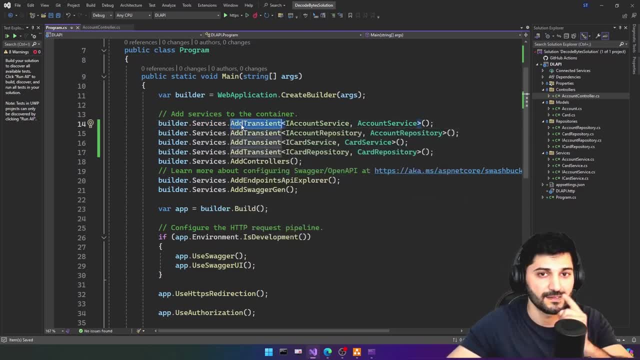 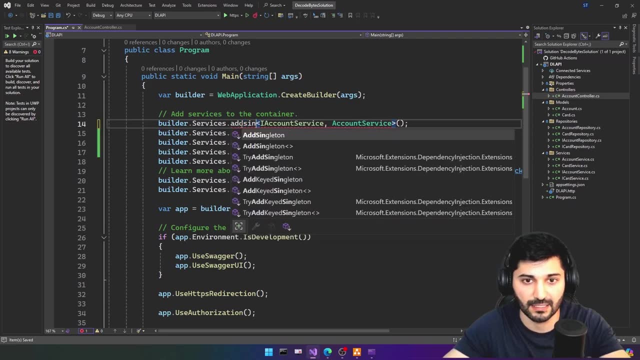 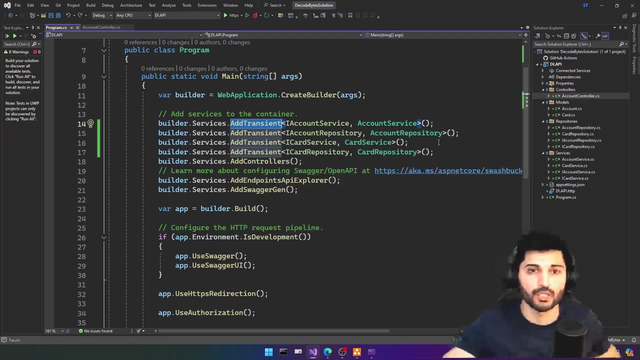 at transient, at service, Scope it and add singleton. You see, we have add scope it here and add singleton here. Just now, focus to implement, to make your application to run successfully, rather than to think about transient, scope it and singleton. Let's run our application. 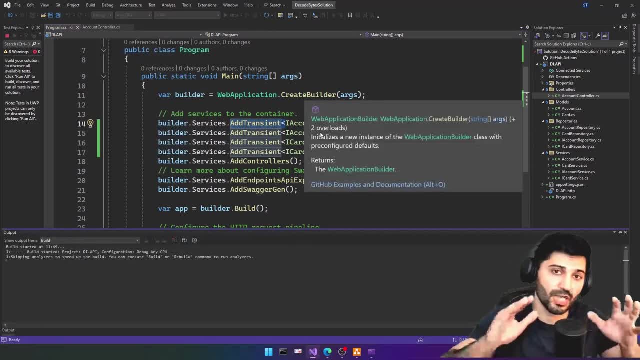 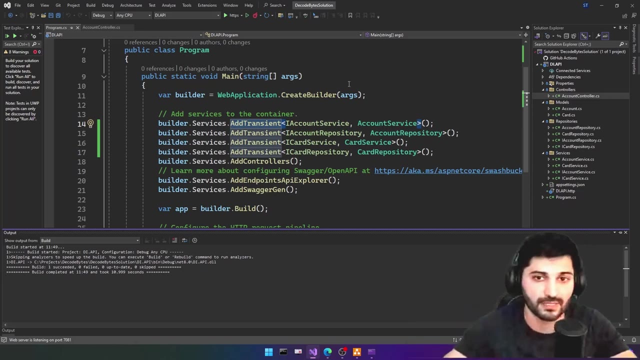 When something is wrong, system will notify that you have this dependency, but you don't have any sync Configure it related to this dependency. So let's see if we are able to run our controller successfully. It means all the cases related to dependency is working. 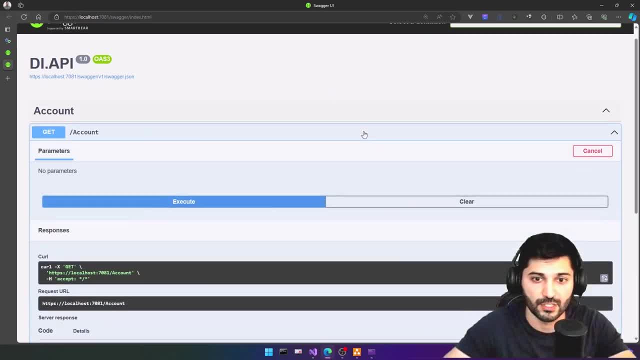 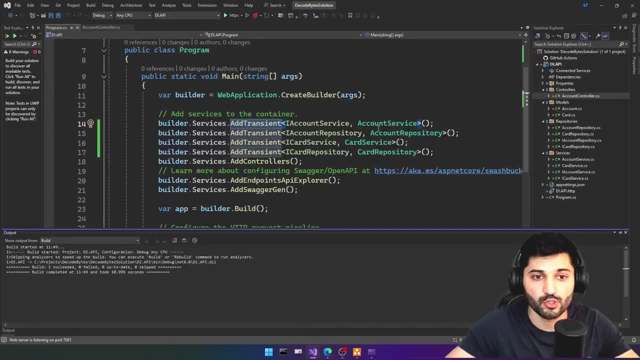 So let me just refresh. Let's go execute And here we are. Everything is working. We are calling our account service And for the account service, we are getting the exact instance of account service, And this account service requires iCard. 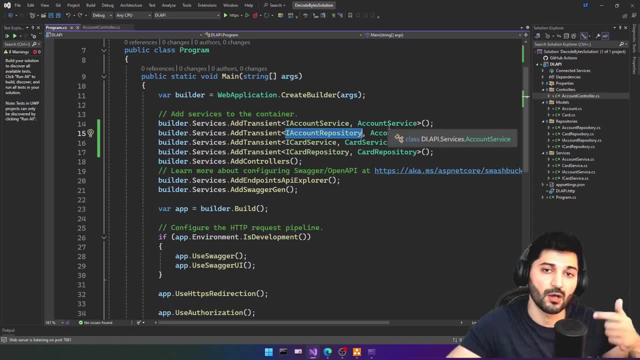 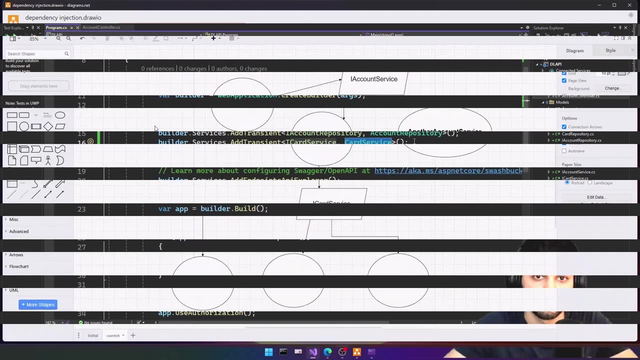 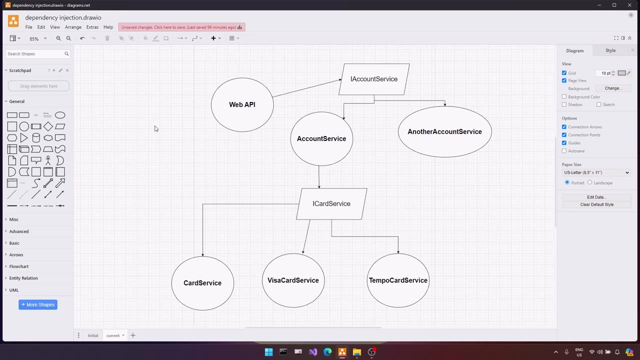 So we are going to call our service and iAccountRepository And our dependency injection container will provide instantiate our objects in a proper manner. I hope I could explain dependency injection as simple as possible for today. That's all from my side. I will have separate topics related to dependency injection, like. 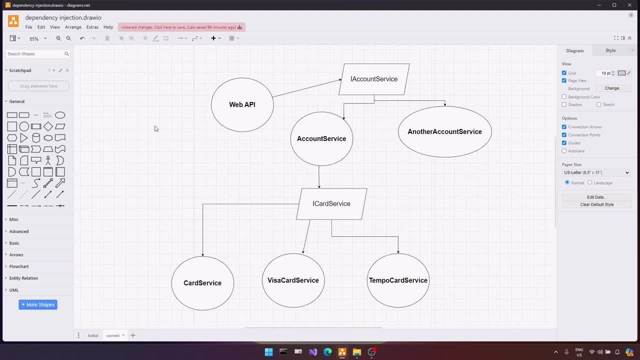 dependency inversion principle. the lifetimes, like singleton, scoped transient. But for now, this is the first tutorial That will help you to understand the basics of dependency injection. If you like my videos, please don't forget to subscribe. hit like button share. And I will see you in the next tutorials. Bye.